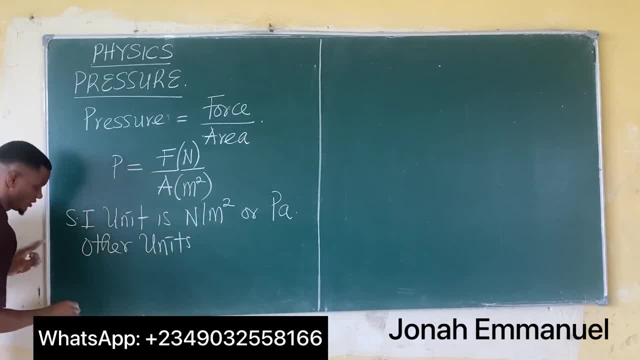 As I mentioned before, S and P reveal each other. You have four units of pressure. So essentially for software, as I said, we are Corner diameter by concept, СТW, displacement 1.0.. 50 as PA, we have VAR and also we have Atmosphere, which is known as ATR. 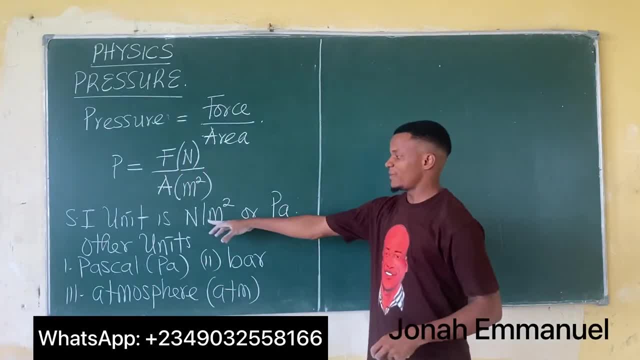 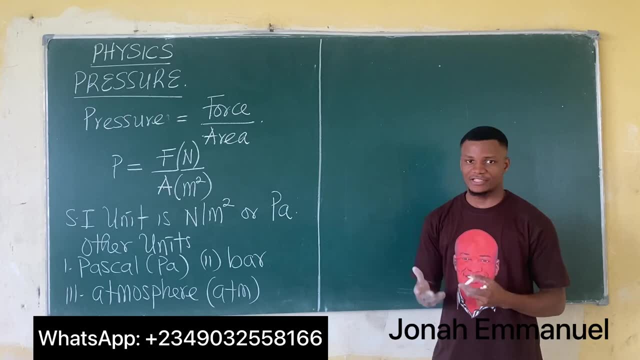 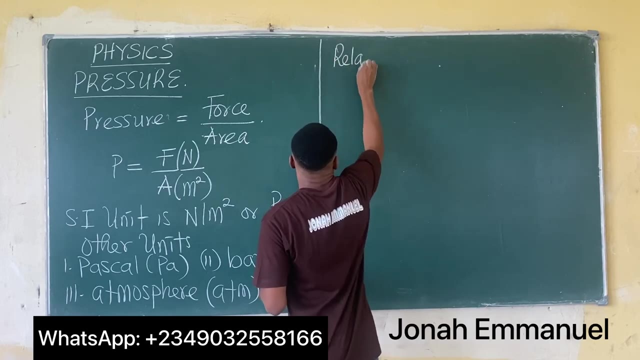 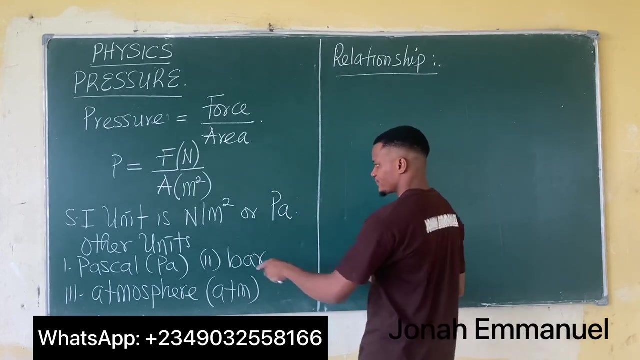 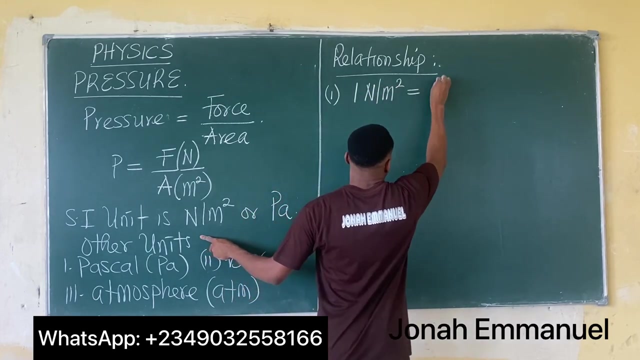 all right, so these are like assigned units per meter square. these are order units for pressure. now the relationship, just in case you want to do a conversion, the relationship for this is that there are one relationship between them is that for the first one, we have that one newton per meter square is equal to: 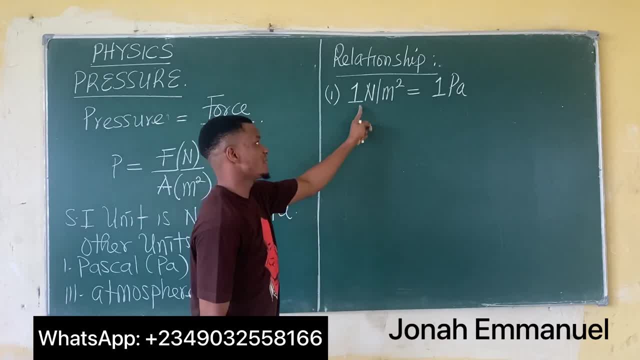 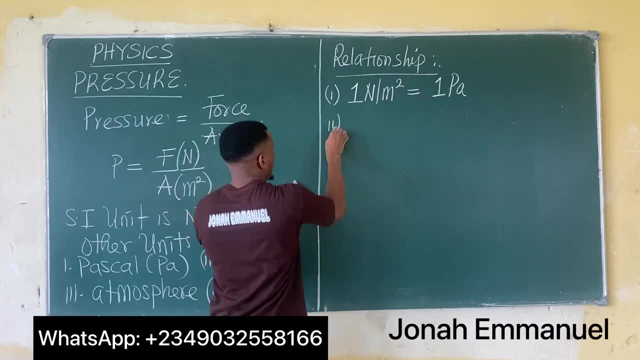 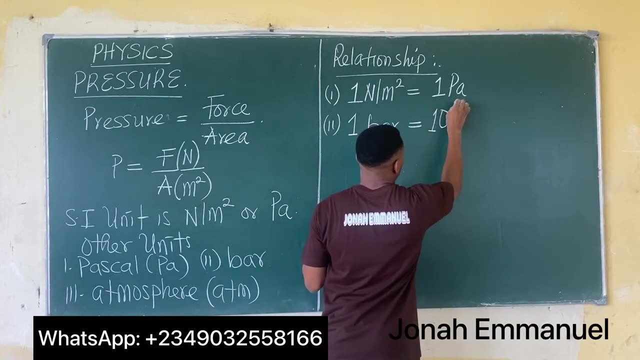 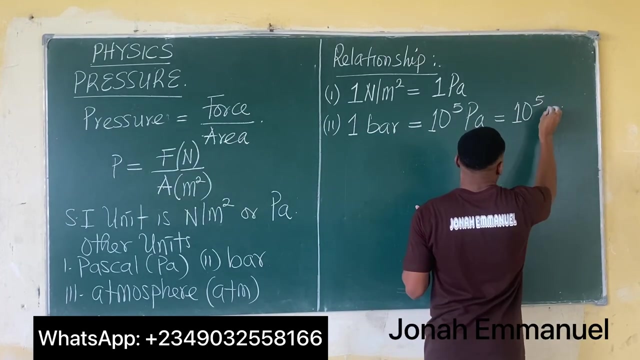 one pascal, in other words newton per meter square, is the same thing as pascal, the same thing. so this is my first relationship. number two: you have that one bar is equal to 10 to the fifth pascal, which is equal to 10 to the 5 newton per meter square. 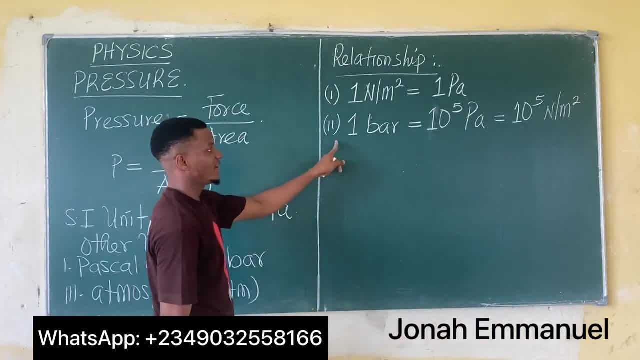 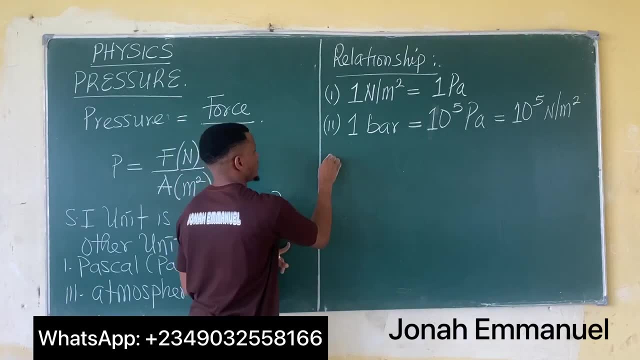 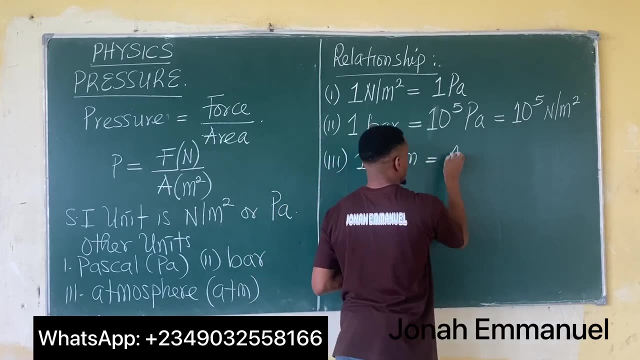 all right. so this becomes the value of one bar one by five pascal, Of course, 10 to the power of 5 meter per meter squared. Number three: we have that one atom square. one atom square is equal to 101, 325 Newton per meter squared. 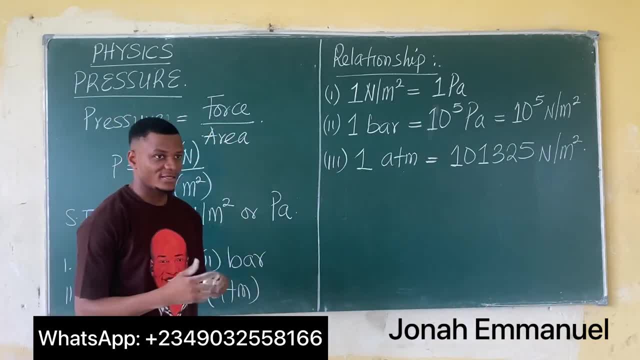 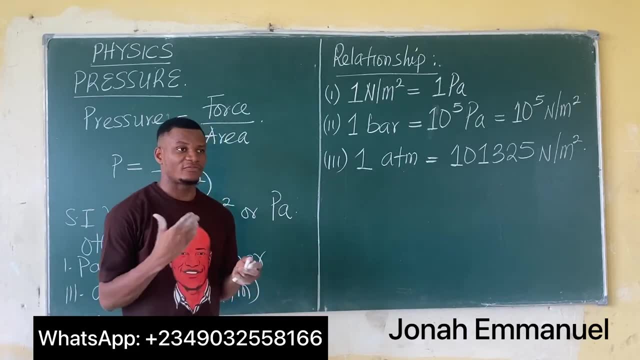 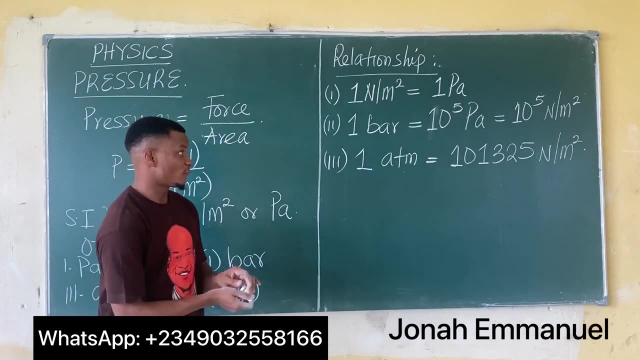 All right, so these are like the way we convert different units of pressure. Aside this, we also have measurement of pressure in terms of millimeter mercury, centimeter mercury centimeter water, etc. but that's above the jam level, So for jam level we just focus on these units. 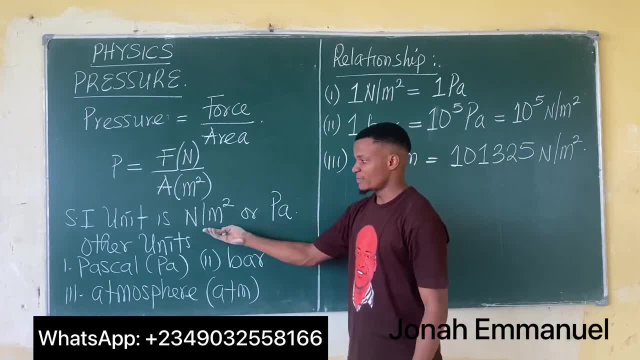 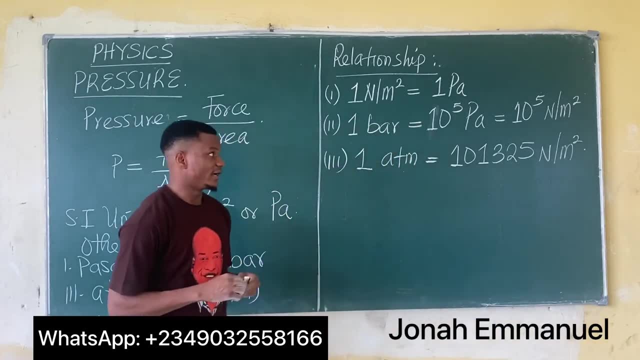 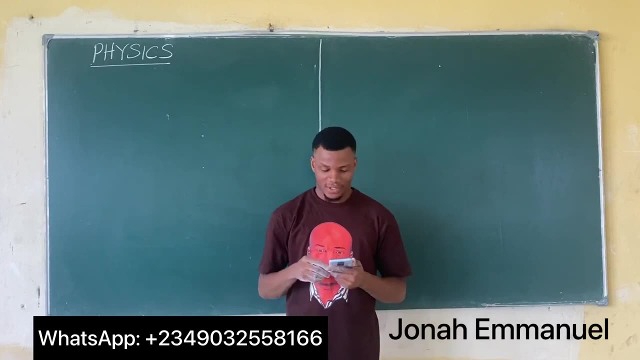 which include Pascal Newton, per meter squared atmosphere and then bar. So these are like the relationship: We take some example and we solve problems together. So let's take the first example. This question says: start with the pressure exerted on the ground. 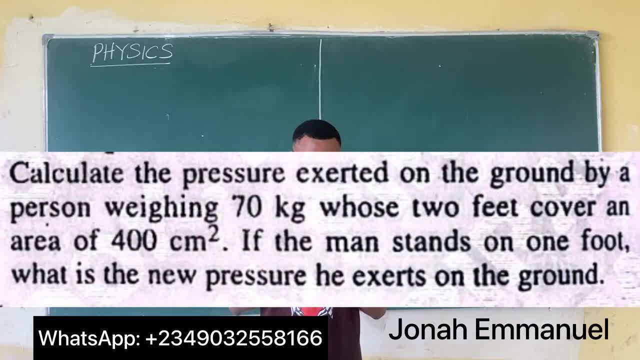 by a person weighing 70 kilogram. Those two feet cover an area of 400 centimeter squared. Who's that? If the man stands on one foot, what is the new pressure he exerts on the ground? All right, so let's get this done. 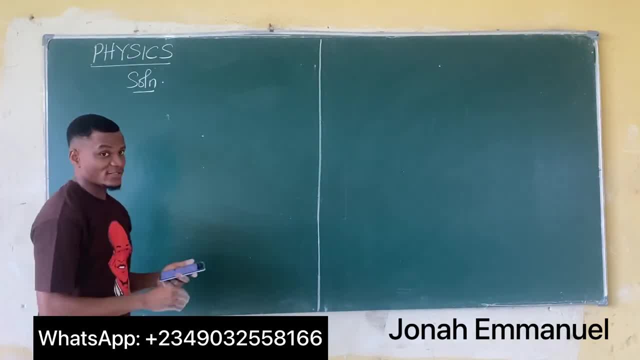 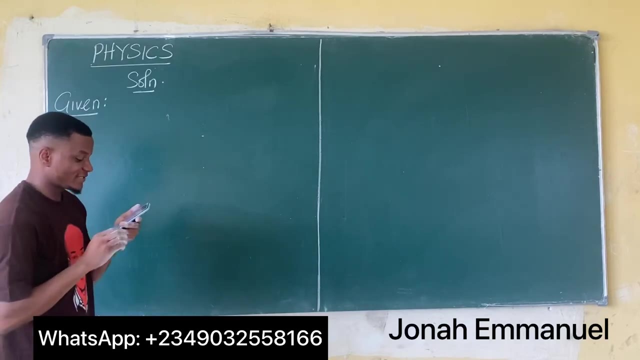 As a solution. as usual, I first start to list out the given parameter. So what are we getting there? So, given going through the question again, it says: calculate the pressure exerted on the ground by a person weighing. the first I'm giving is the weight. 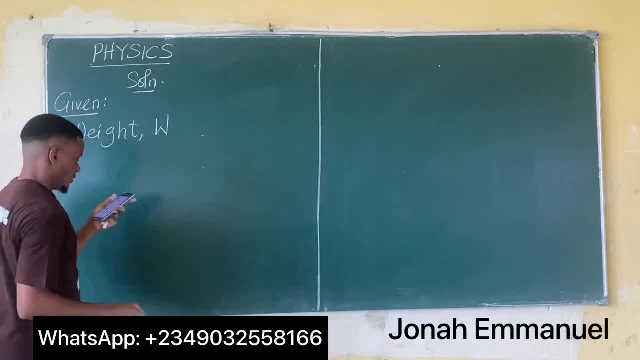 of the person, that's W, But observe that the weight is given as 70 kilogram. Of course, kilogram signifies mass, so instead of weight actually going there mass, weight actually going there mass. So, instead of weight actually going there, mass. 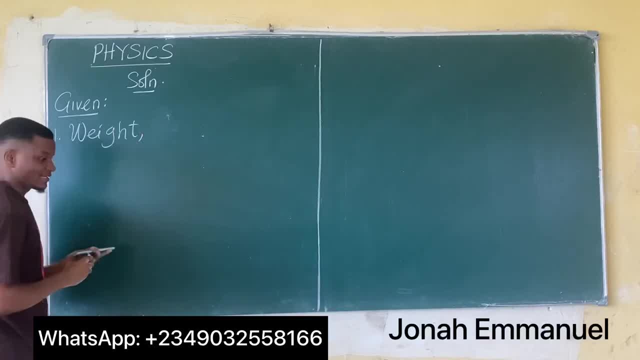 so instead of weight actually going there, mass. so hence I'm giving the mass, not the weight. So I'll just change that to mass, that's N as being 70 kilogram And this is kg 70 kilogram. 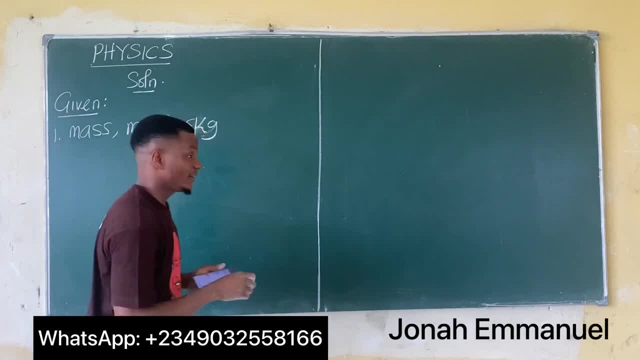 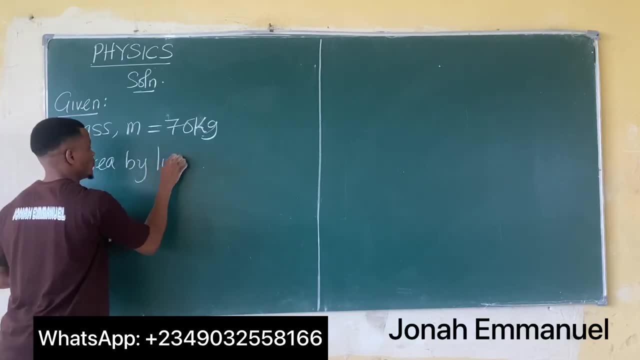 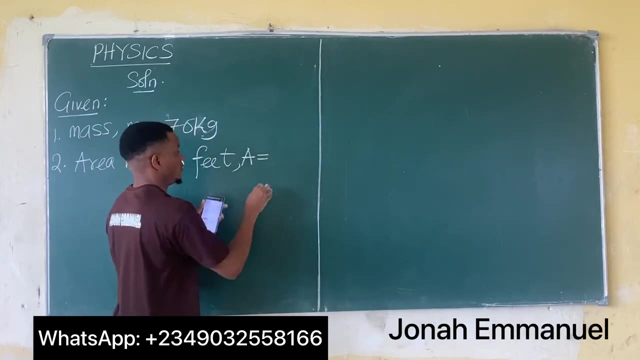 Now the question is: who's two feet cover an area? number two: the area covered by two feet, area by two feet is that's: A is equal to the same 400 cm squared, 400 cm squared. so I have this. 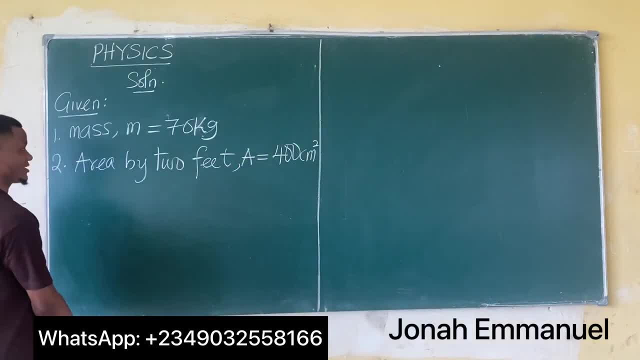 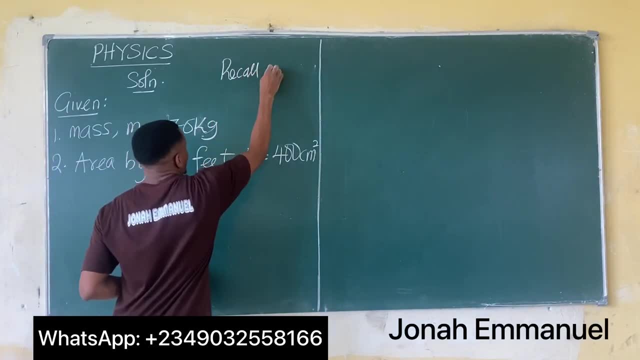 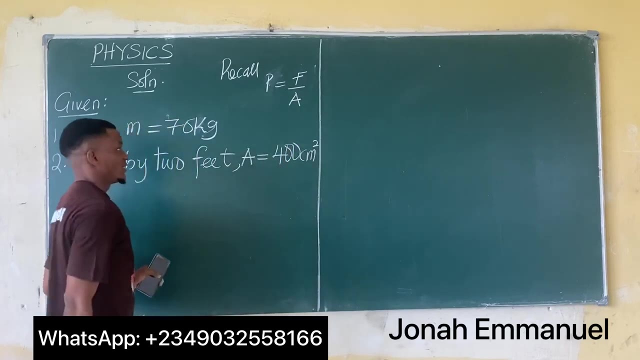 All right. so first of all, we have to find the pressure that this man exerts. Now recall, recall that we said. recall that we said force or pressure is equal to the weight of force over area, And we said from two second of motion. 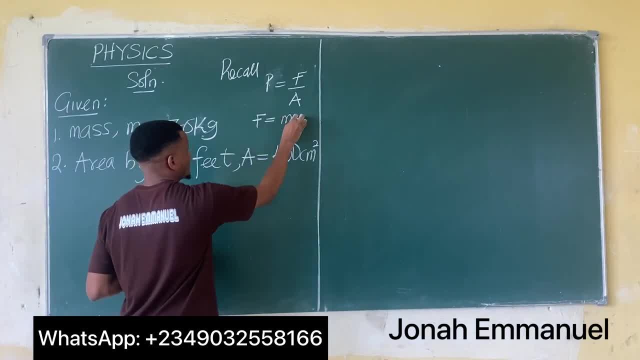 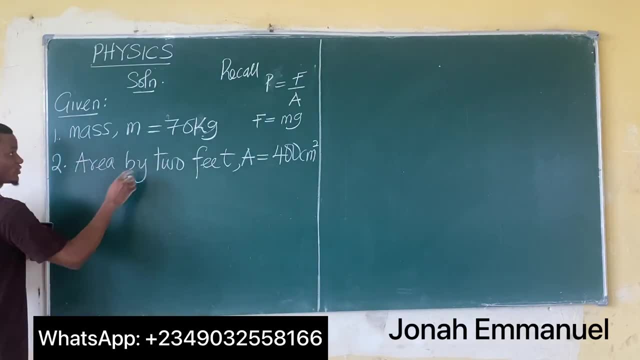 we can say: force is equal to mass times, acceleration through acceleration of, perhaps, gravity, if you want to. So in this case, lets get force. so first let's get force. We said, recall that force F is equal to mass times gravity, And that's equal to mass is 70 kg times gravity. 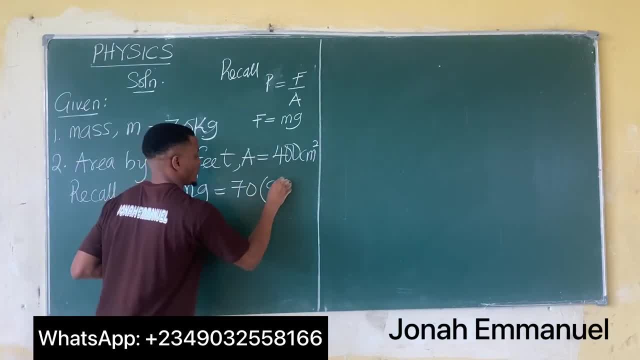 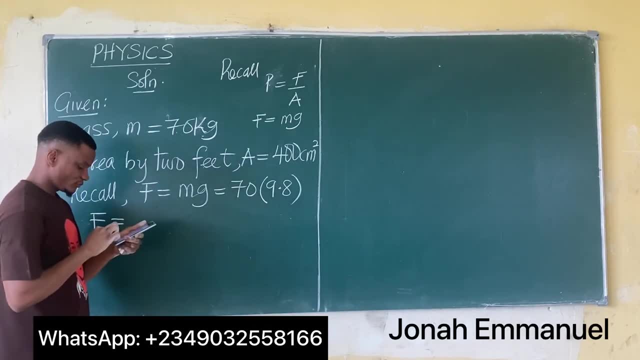 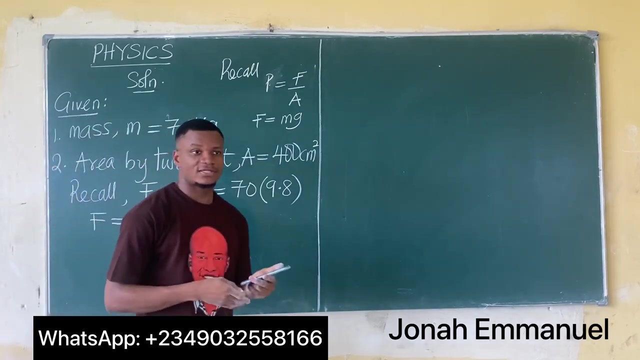 but we said to push fearless. I can put times: gravity is about 9.8 times the constant. so that means the force is equal to, let's say this, 70 times 9.8. 70 times 9.8, that is about 686 in newton. all right, so that means the weight is 686 newton. 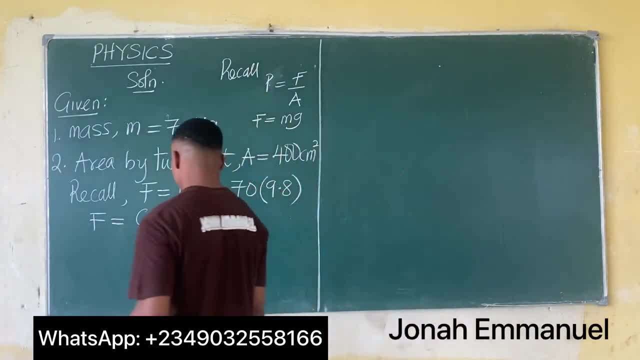 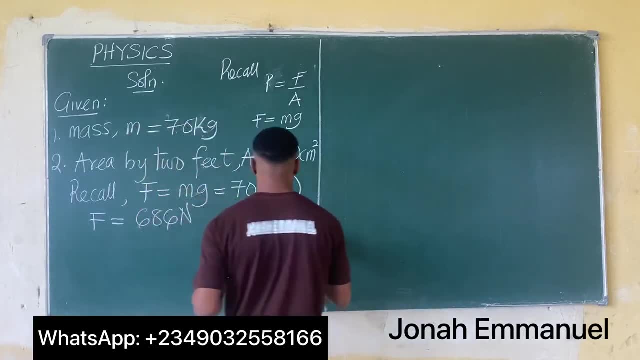 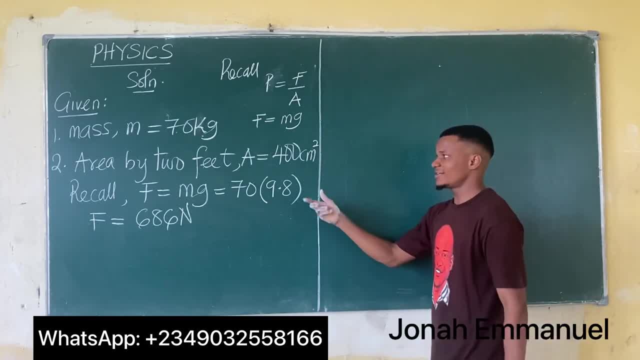 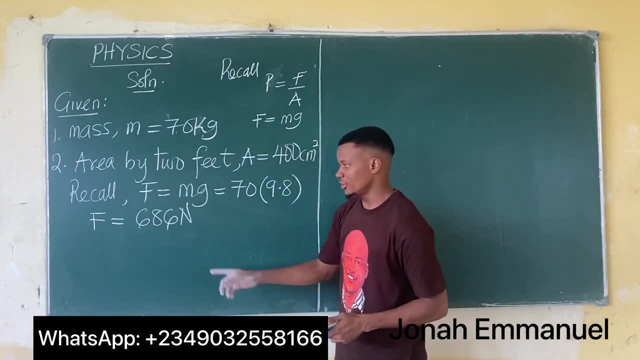 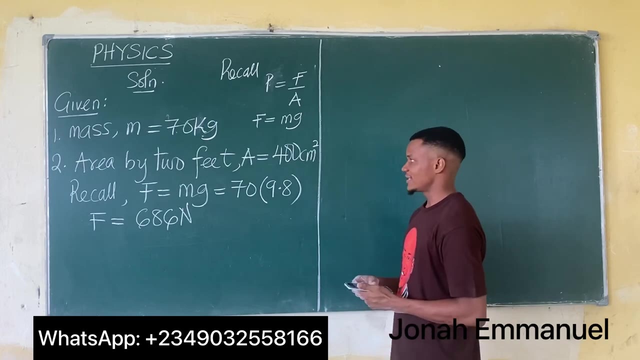 from cm squared to what meter squared? of course you can see the area as cm squared, and so if i solve this way, my pressure will measure in newton per cm squared. that's centimeter square, but let's convert the meters. so the question is this: if i'm to convert from centimeters to 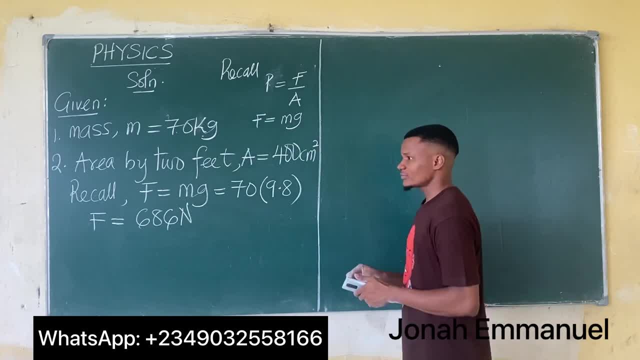 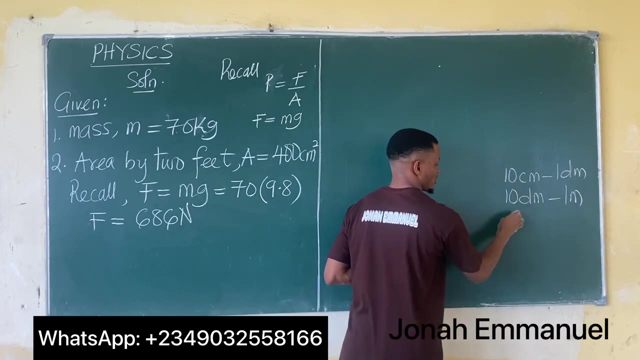 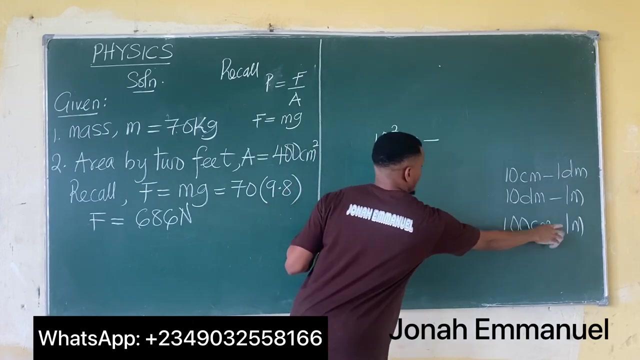 meter. what do i do now? here's what to do. if i record the relation, it says: 10 centimeter makes one decimeter, 10 decimeter makes 1 meter. So from here to here it comes here: 1, 2, 2 zeros Cm makes 1 meter. So I'm having this here. If I express this in index of 100 is 10 to the power 2 centimeters gives you this, one here is 1 meter. 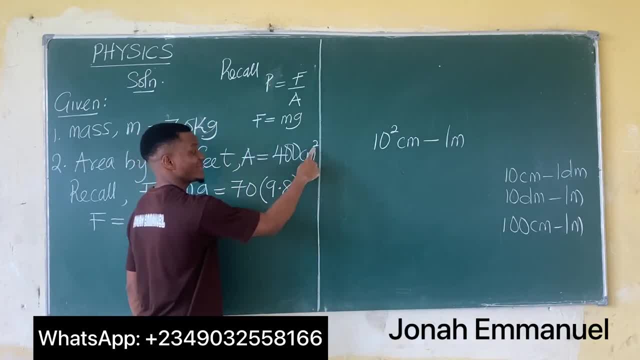 But observe, I'm having to convert between centimeter square and not just centimeter. This is where we make mistake. If you want to convert from centimeter square to meter, you go dividing by or multiplying by 100. That's not the case. 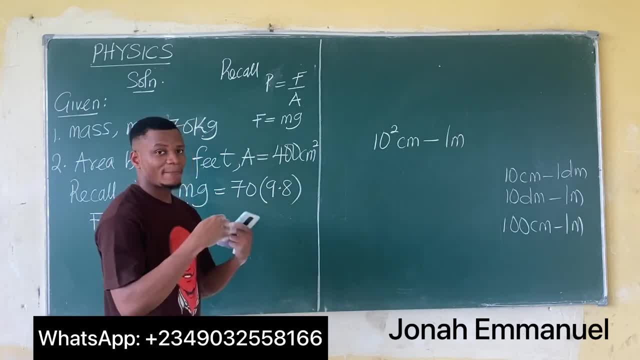 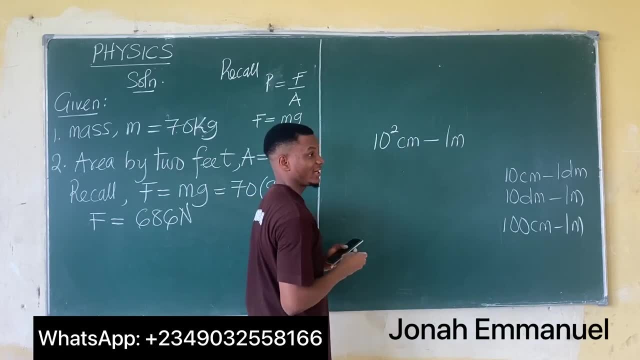 So my first case has to be getting the proper relation between: observe: Cm square, not Cm. So if I'm having Cm here centimeter, I want to get Cm square, What do I do? So I'm having Cm here centimeter, I want to get Cm square, what do I do? 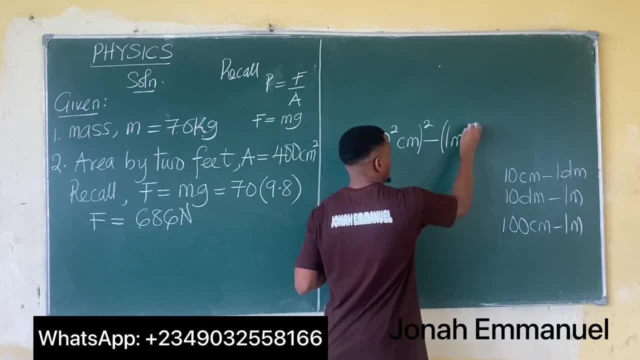 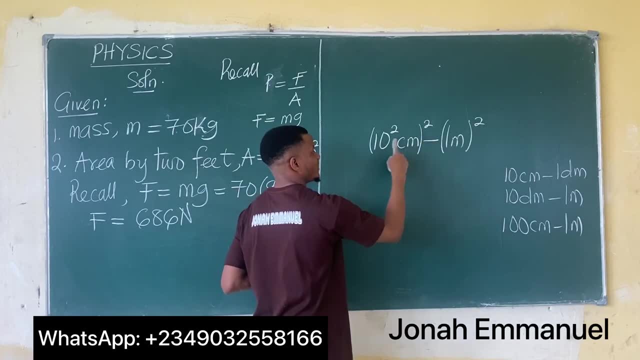 This is simply putting square here compared to square this. So I have to square both sides. Is that simple? So these two multiply From the idea of indices, this becomes 10 into these two. multiply 2 times 2 gives you 4.. Then Cm square. 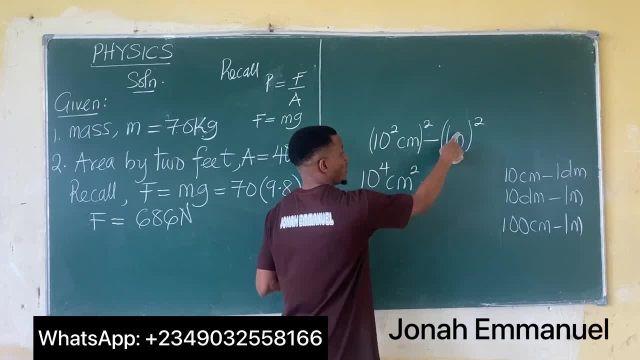 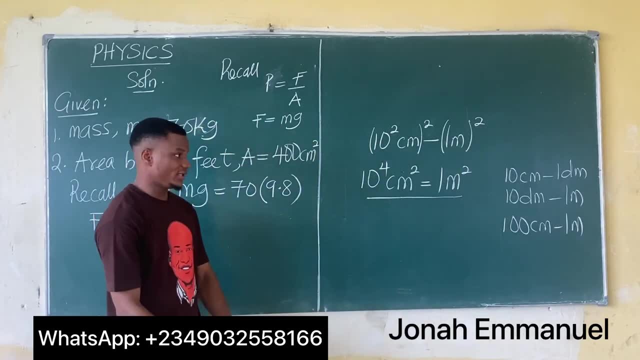 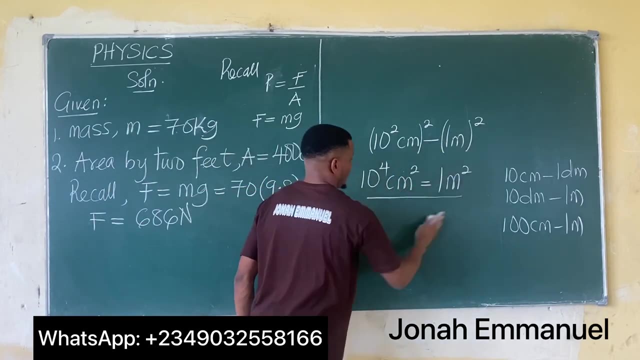 So Cm square is equal to 1, square is 1.. Then meter square. This becomes the proper relation between Cm square And meter square. So we have this All right. So this becomes the relationship here. The next task will just be bring this on that here. 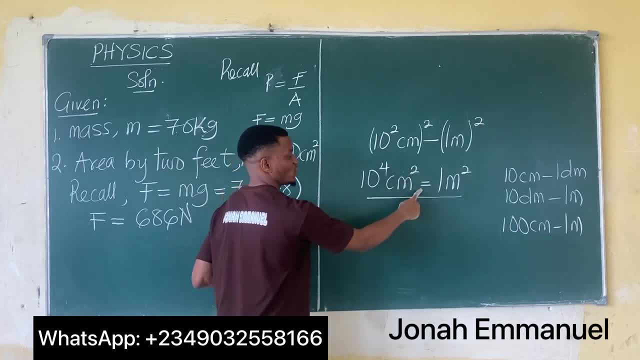 So if 10 to the power, 4 Cm square gives you 1 meter square, how many meter square? let's call this? x will be equal to what I have here: 400 Cm square. Now, this is like the basis of conversion. All right, For the basis of conversion, first of all, get the relationship between the two parameters in conversion. 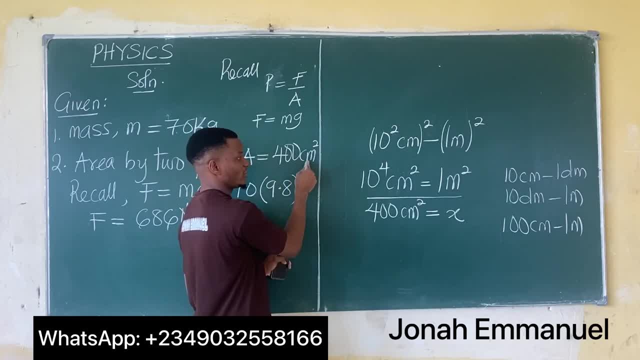 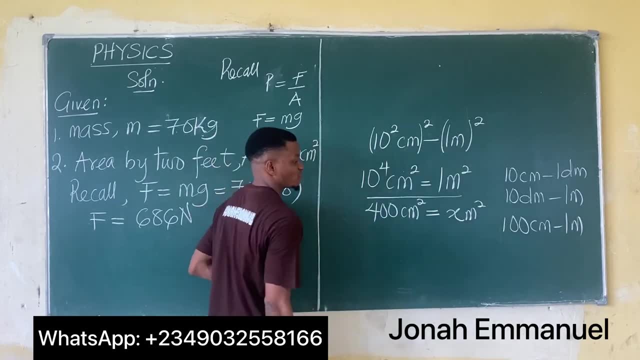 Next up, bring me what I have here: 400 under Cm square, that's this. Then an unknown value under meter square. Here we cross. multiply This times, this, this times, this, So this times, gives you 10 to the power. 4 times x is equal to 400 times 1.. 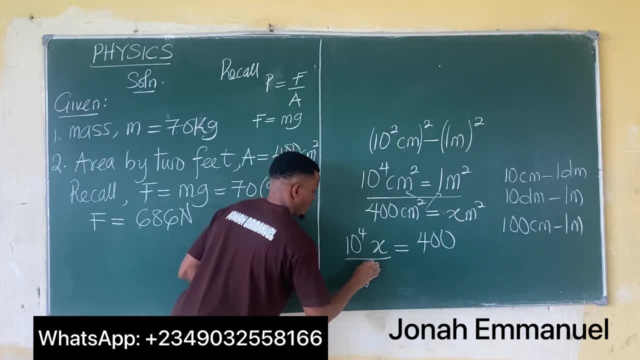 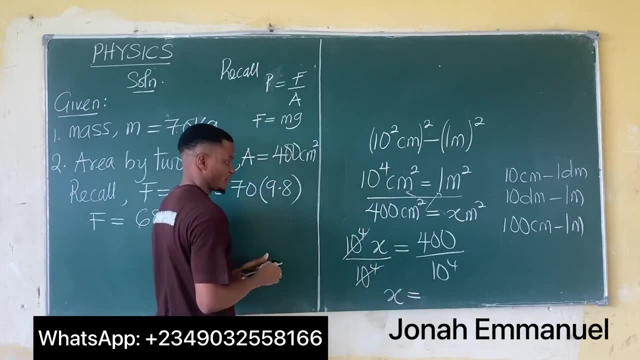 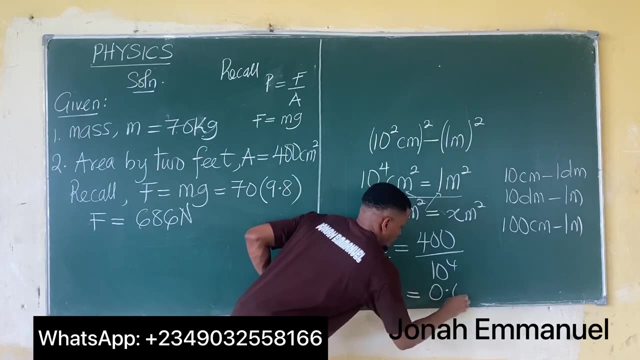 That's 400.. Divide here by 10 to the power 4.. Divide here by 10 to the power 4.. I will have that x Is equal to Lester's division 400 divided by 10 to the power 4.. That gives you 0.04 meter square. 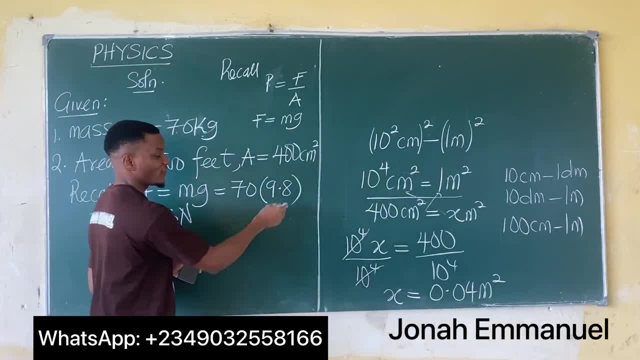 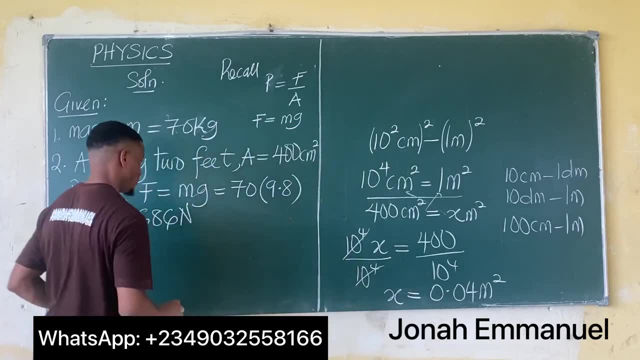 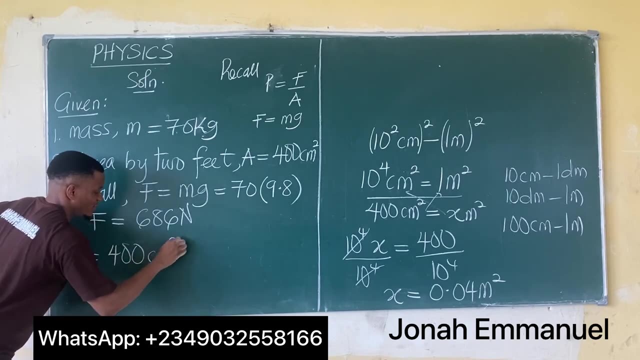 So you have this. So, in other words, to convert from Cm square to meter square, simply divide this value by 10 to the power 4.. That's all. So area giving us 400 Cm square is equal to 1.. 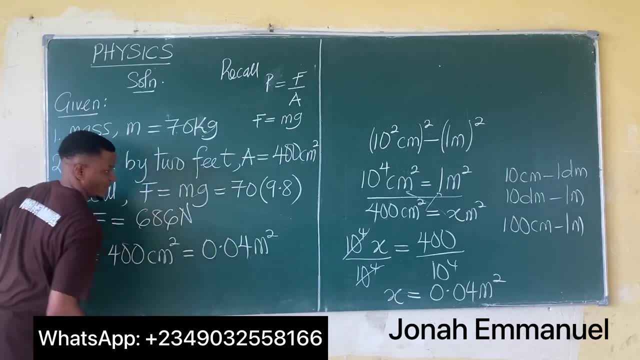 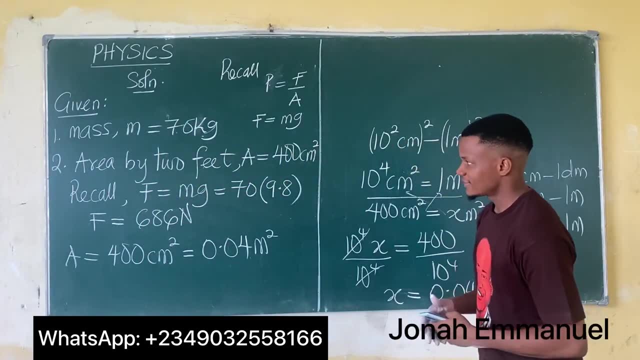 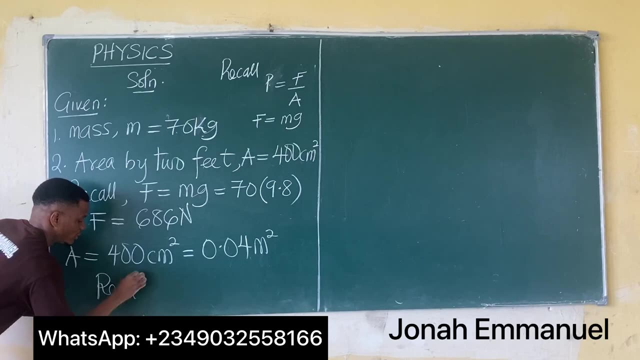 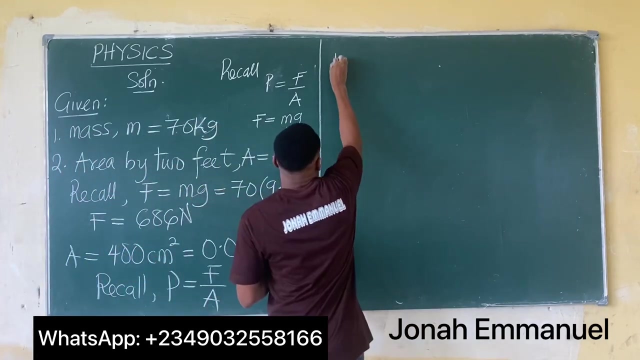 0.04 m2. so I have this alright from here. now. we can now get the pressure exerted by the man's feet. alright, so from here I recall that we said pressure is equal to force all over area. so we have that: pressure is equal to force. 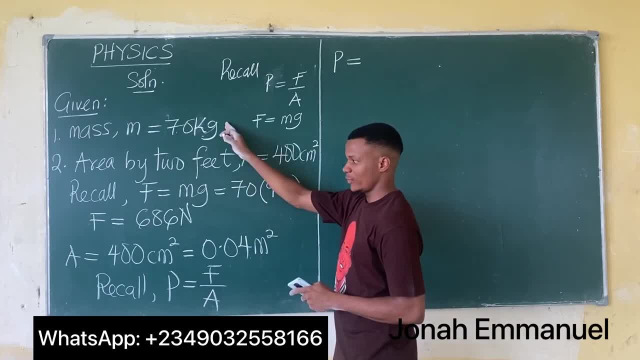 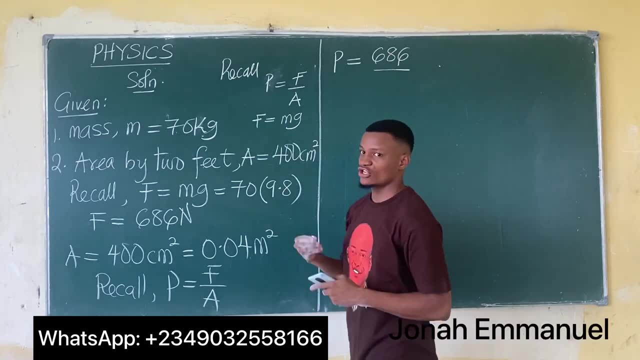 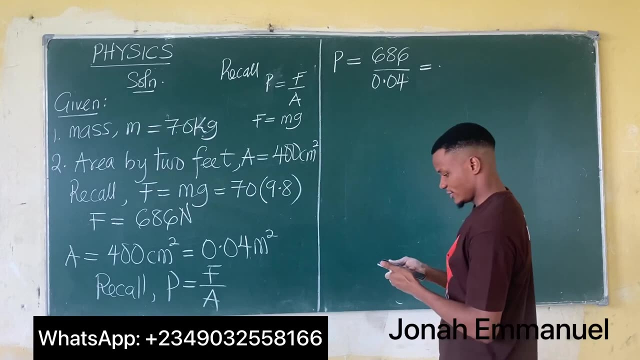 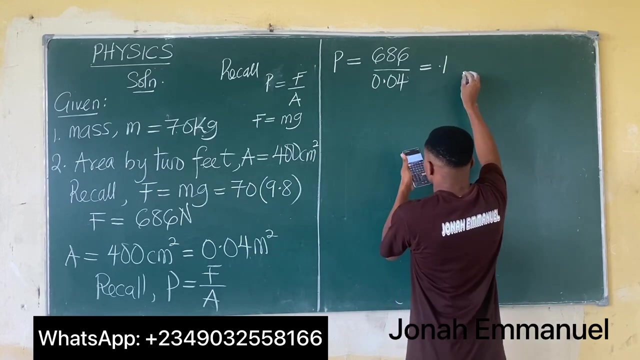 or which is, in this case, like I said, weight. that's equal to 686 all over area, which we have successfully compared to m2 as 0.04, and that's equal to 686 over 0.04, that's about 17150. 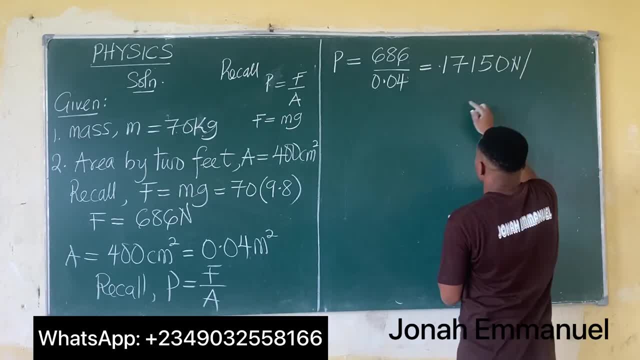 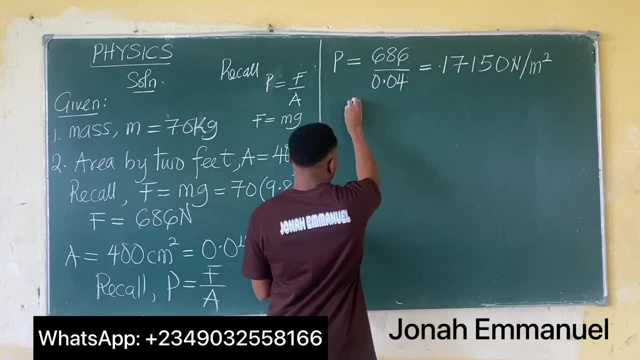 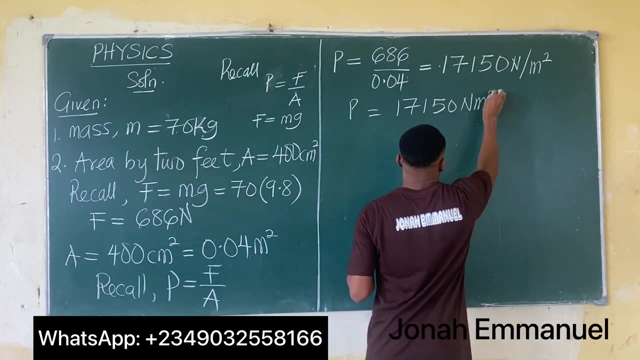 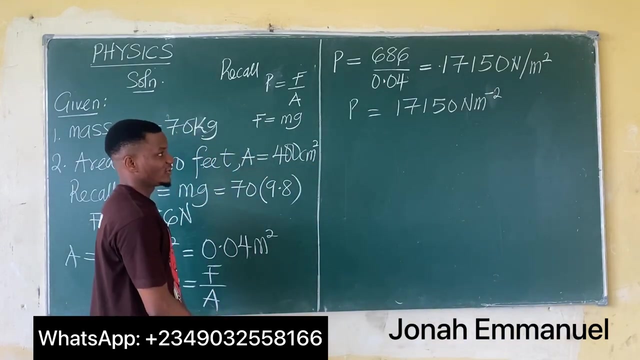 this was in kelvin. all over this was in m2, so I'm having this value. ok, so to that end, the pressure is equal to 17150 Newton per m2. Newton per m2 or Pascal, whichever one I have. so this is the pressure you can do the conversion from here. 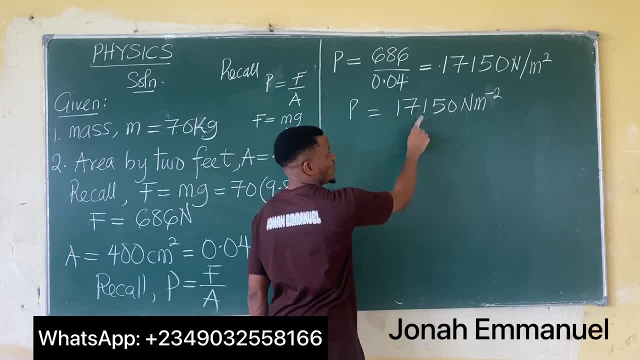 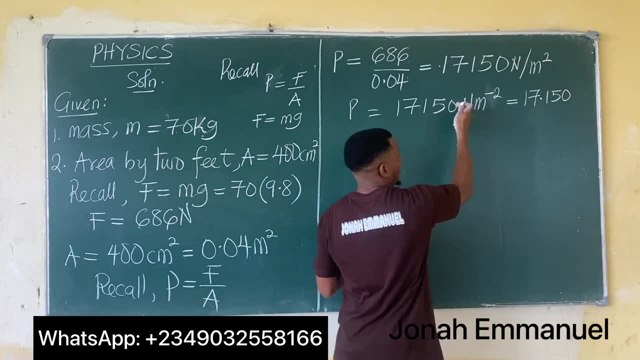 you can take 1,, 2,, 3,, so it becomes 17.15 kN, that's equal to 17.15m2. from here, if I move 3 times backwards- 1,, 2,, 3,, 17.15 becomes a kilo. 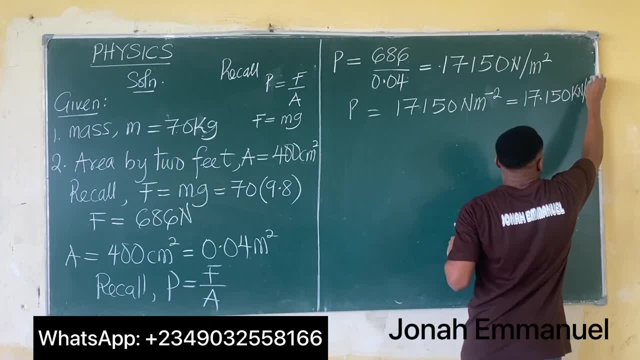 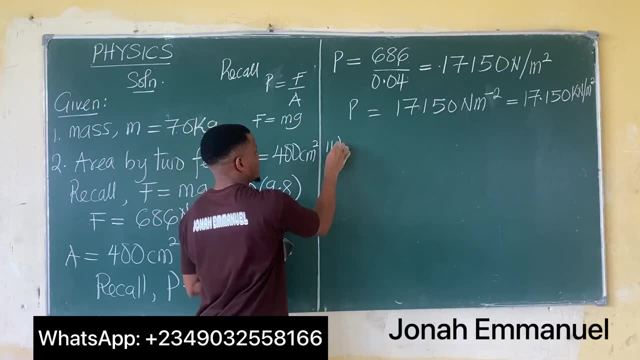 kilo newton per meter square. so I have this, whichever one works. so this is my answer. the second part of that question says something. the second part says what is the new pressure? we said if the man stands on one foot, what is the new pressure he exerts on the ground? 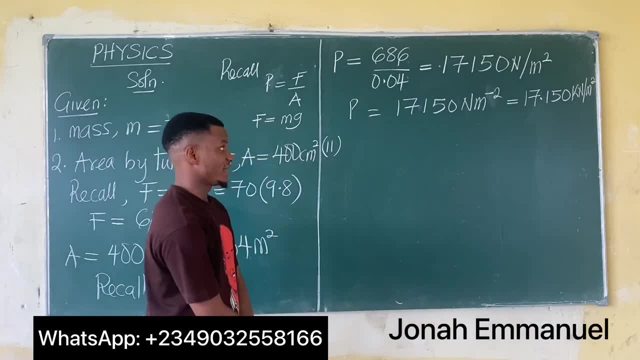 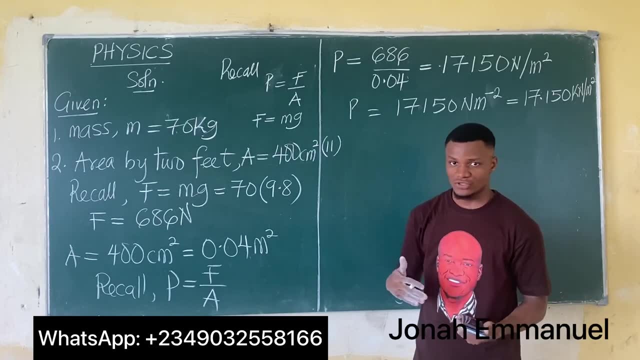 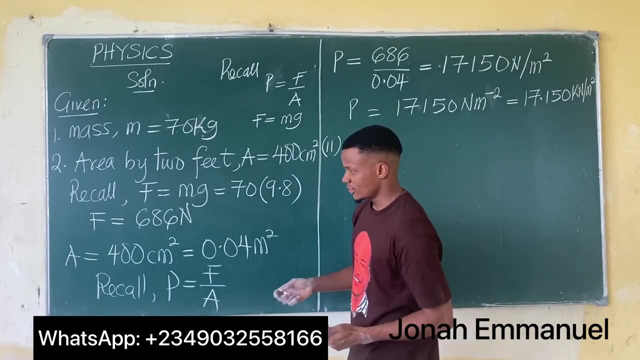 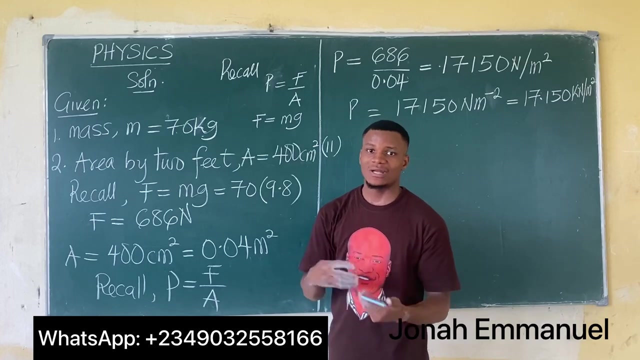 if he stands on one foot, what is the new pressure he exacts on the ground? the question will now be: which of these parameters does his foot influence? all right, the parameter that the foot influences is what the area. of course, the foot will occupy a particular space on the ground which is also over there, a particular area of the ground. 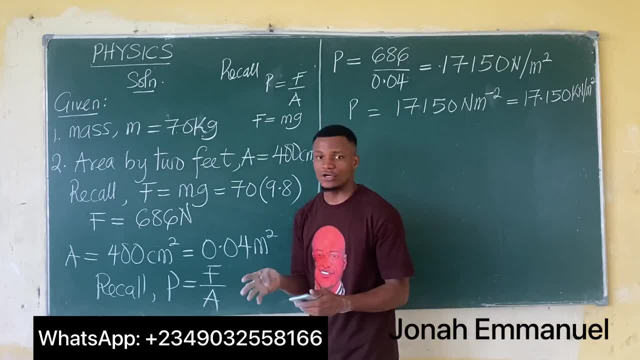 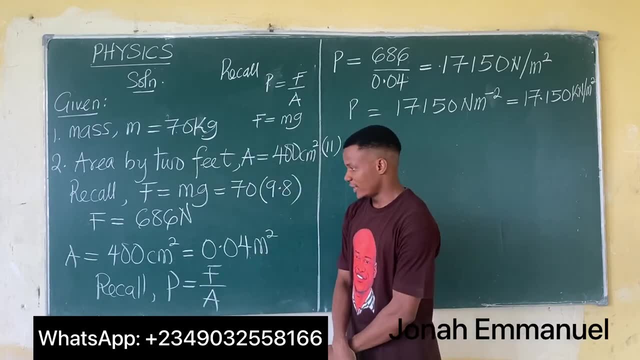 all right. so if that's the case, that means if he stands on his feet, that's both, uh, both legs there. he will occupy 400 cm squared, which is 0.04 meter squared. what if he now stands on just one foot? he will occupy half of this. so hence, standing on one foot would mean, uh the area, because 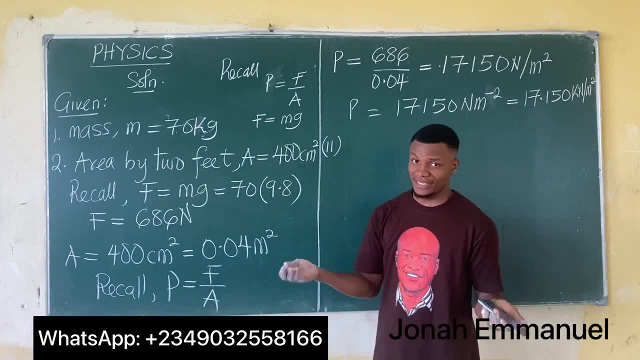 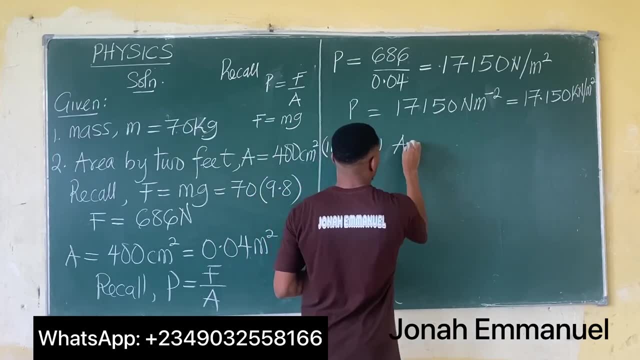 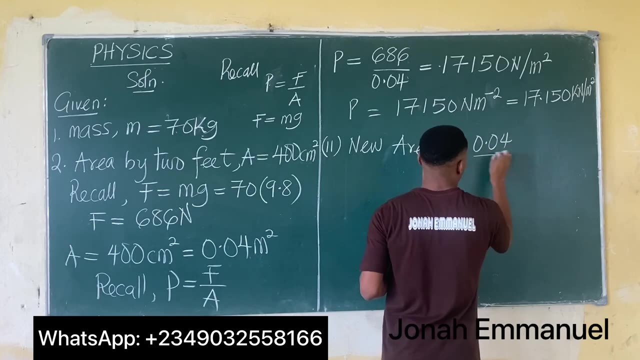 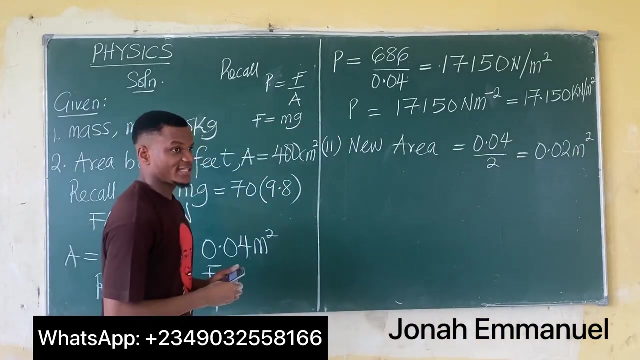 of the half of the total value. of course, it has two legs, so if that is true, that means the new area. the new area is equal to 0.04 all over 2, that's 0.02 meter squared. it's just a simple logic. he stands on his feet- that's both legs, and he occupies 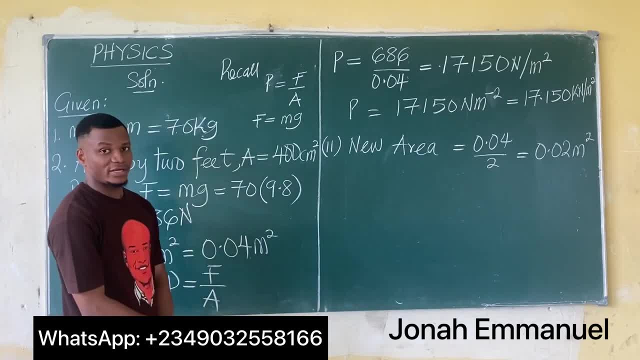 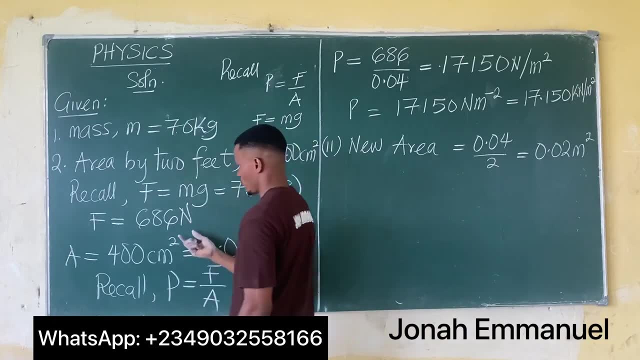 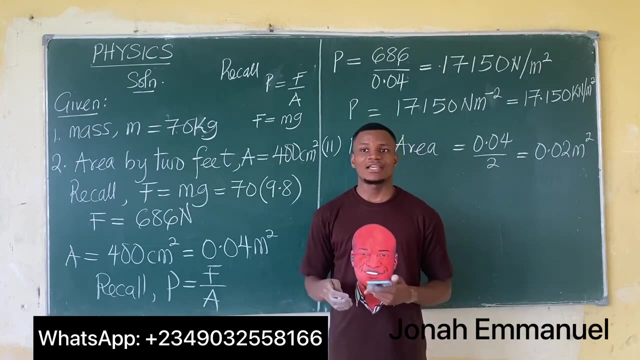 0.04 meter squared. so if he stands on just one leg or in foot, of course becomes half of the total area, which is this. but will he wait or will he force exacting the force? if the force is exacting, won't it be affected? of course not, in fact. this is why, if you stand on just 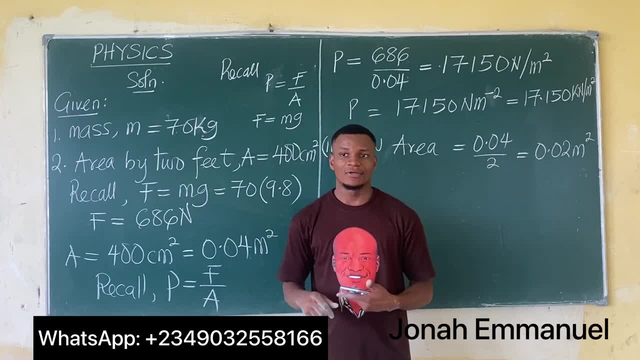 one foot for long, begin to feel tired. why? because the weight that was shed by both feet is now being shed by just one foot, so the same force will apply and because of that, one foot is carrying the entire weight. that's why, if you stand on just one feet there, 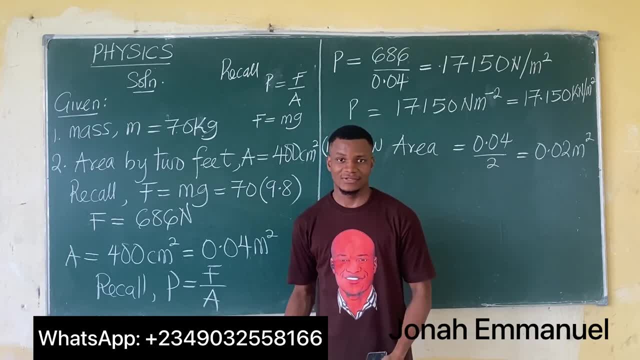 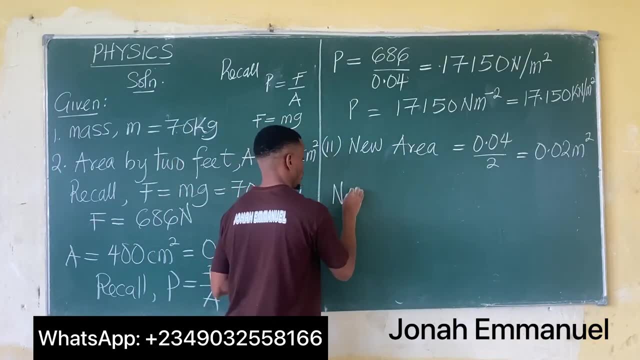 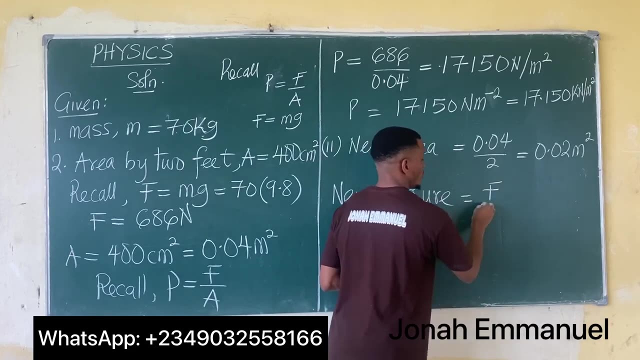 you need to feel pressure of that leg becomes tired. so that's the simple analogy there. so you know that was the force would not be affected. so hence the new pressure. the new pressure is equal to the same force all over the new area. let's call this a2 if you have to, so all over a2. 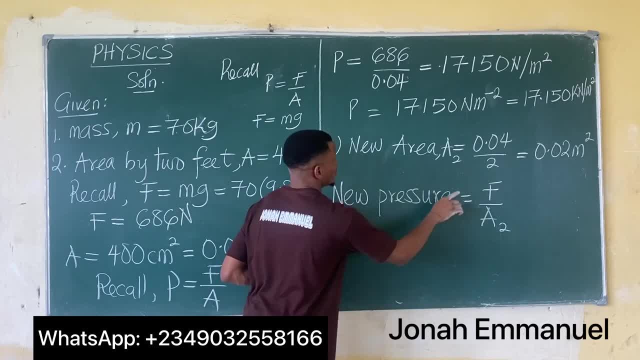 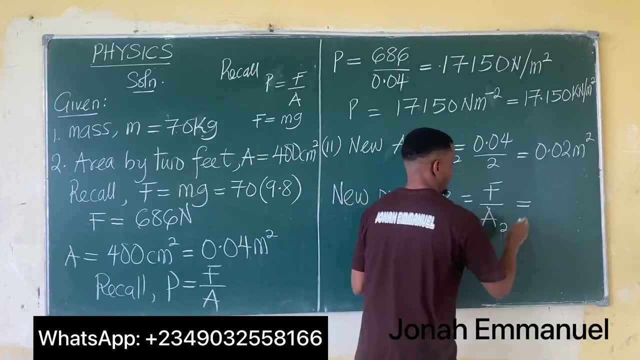 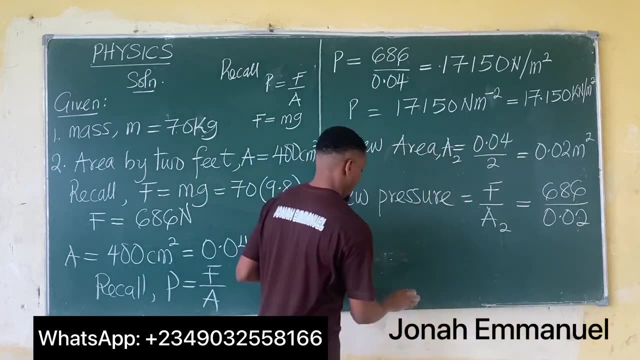 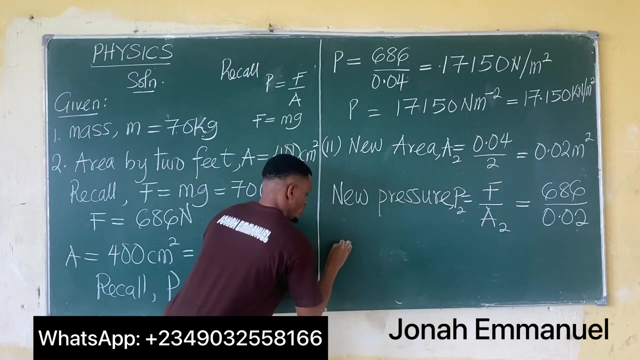 so the new pressure is equal to the new force. so equal to the force. the force is 686, 686 all over the new area: 0.02. hence the new pressure. so let's call new pressure, let's call it p2. perhaps p2 we'll have that p2 is equal to 686. 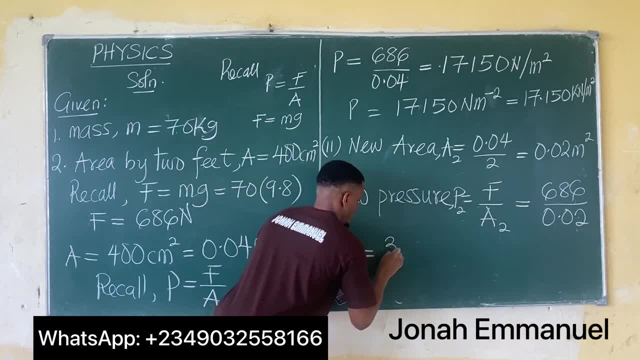 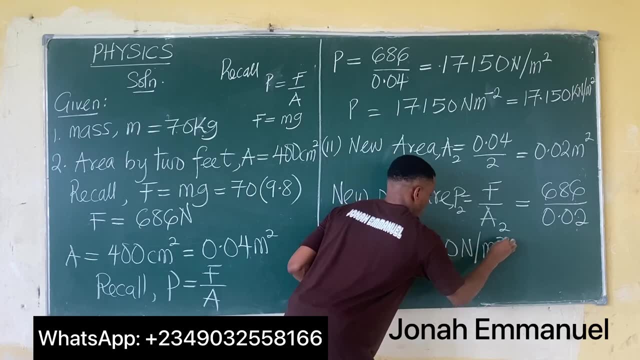 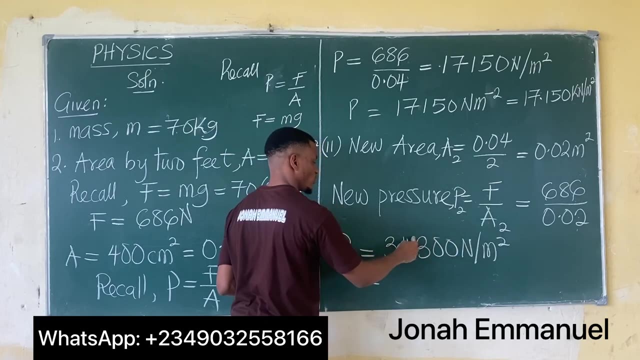 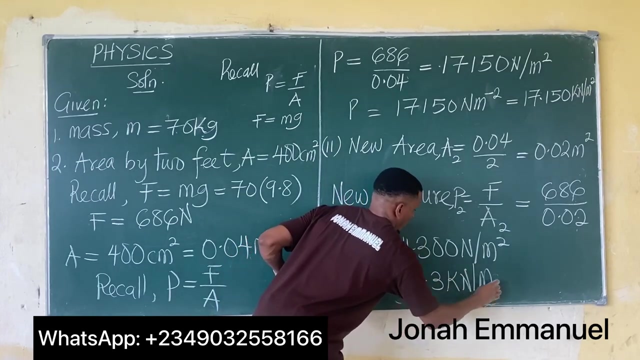 0.02, that's about 34 300 in newton force all over area meter squared. if you want to combine this to kill you. so what do we do from here? move backwards three times: one, two, three, so it becomes 34.3 kilo newton per meter square. all right, so this is how we solve this. 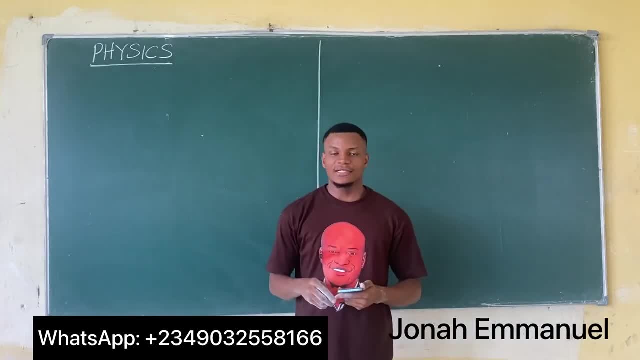 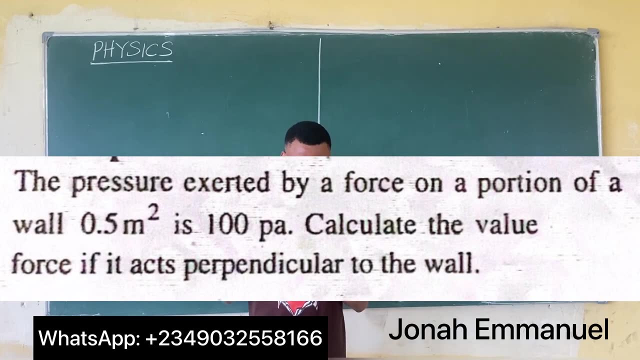 question. Alright, so let's take a second example. This question says the pressure exerted by a force on a portion of a wall, 0.5 meter square, is 100, Pascal as VA. Calculate the value of the force if it acts perpendicular to the wall. 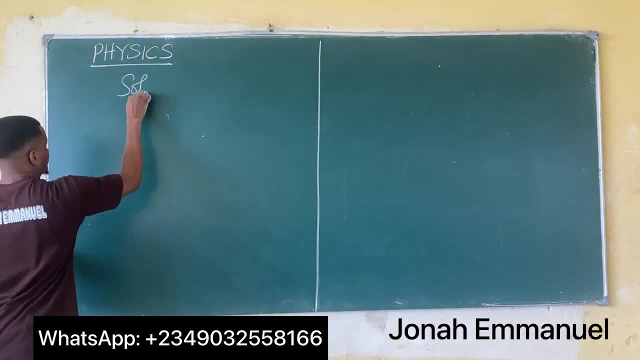 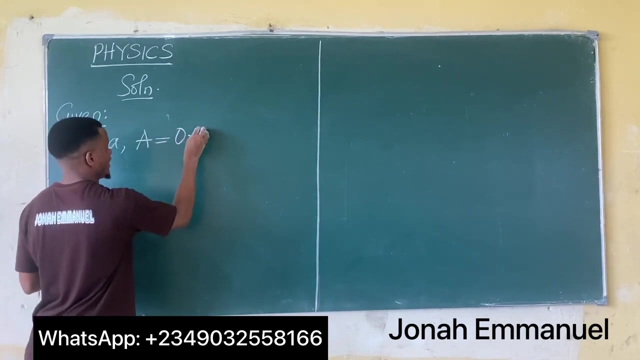 Alright, the solution is So let's get this done. Solution as usual. Let's list out the different parameters. So the first thing that it says: calculating pressure exerted by a force on a portion of a wall: 0.5 meter square. So because I'm seeing meter square there, it tells you that that's area. So area is 0.5.. Area is 0.5 meter square. 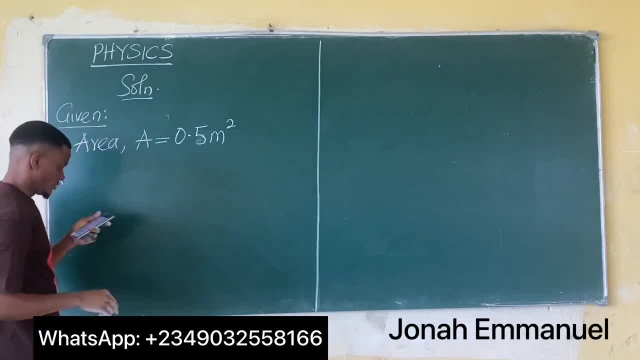 They said the pressure is 100 Pascal. Pascal is pressure, So pressure P is equal to 100 Pascal. Alright, we have to find what there Calculate the value of the force. We have to find force F equal to unknown. Alright, let's get familiar. 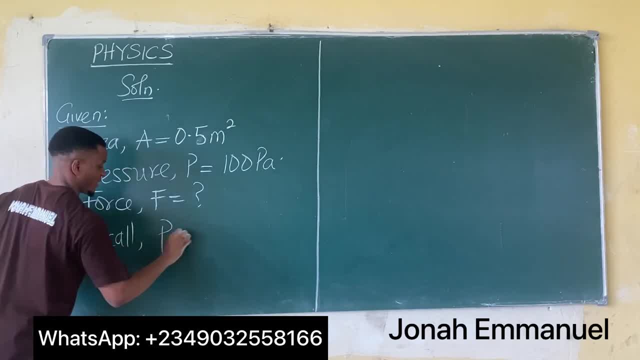 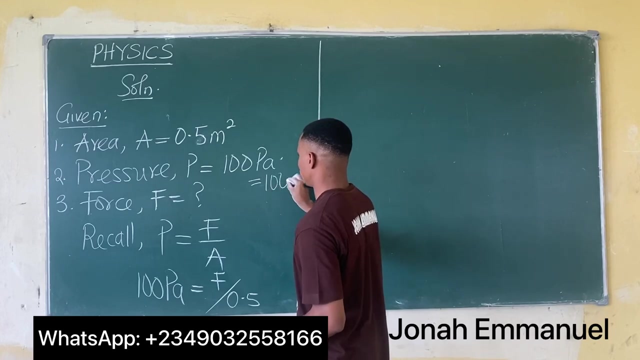 So recall, Recall that we said pressure is equal to force over area. The pressure here is 100. Pascal is equal to my unknown force all over The area is 0.5.. Observe that all of these are in their basic units. Pascal, we said, is the same thing as 100 Pascal Newton per meter square. In other words, I don't have to. 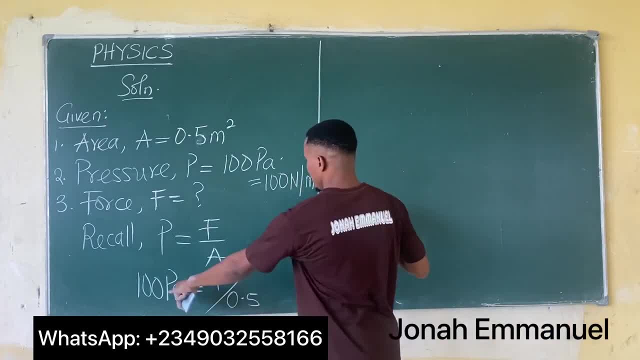 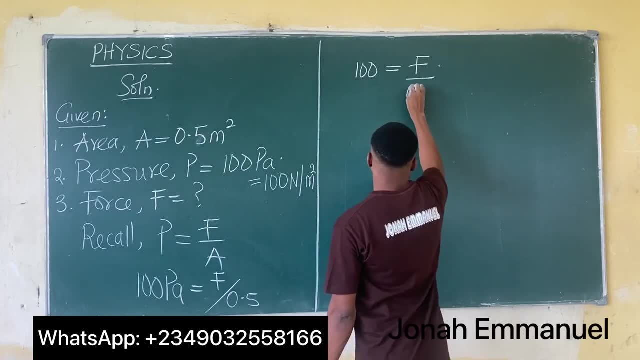 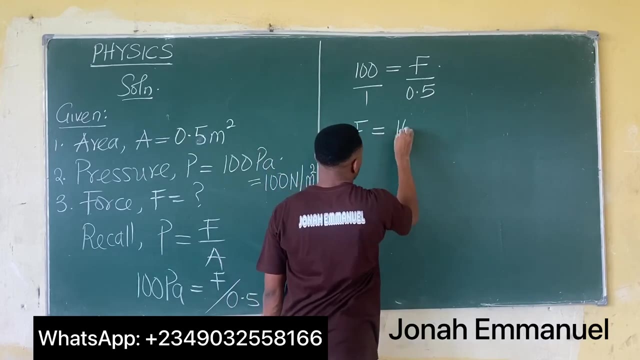 convert again. So hence, from here, I'll be having that 100 is equal to force all over 0.5 over 1.. Cross multiply Force times 1.. Force equal to 100 times 0.5.. Alright, If I work this out, I'll have that force is equal to 100 times 0.5.. Simply means half of 100.. And that's. 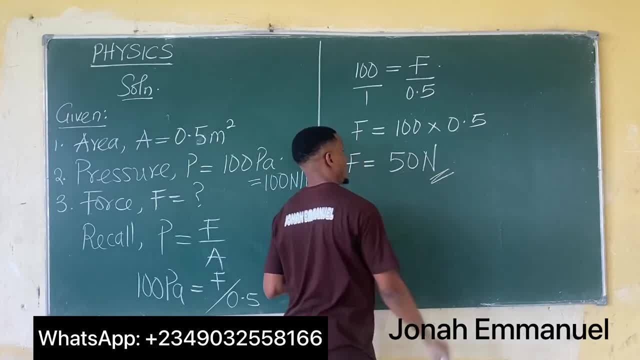 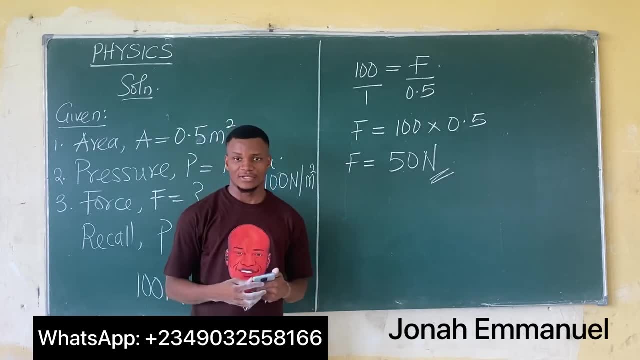 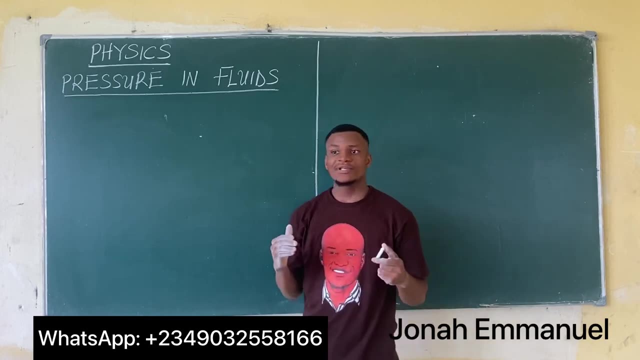 equal to 50 Newton. Hence, the force required is 50 Newton. So this is how you solve this question, Alright. so let's look at our next task, That's pressure in fluids. Alright, What we discussed earlier about pressure was simply pressure for solids. Alright, And that's why, if you look at the second example, it said something about a wall. It talked about a wall, which is what A solid body. 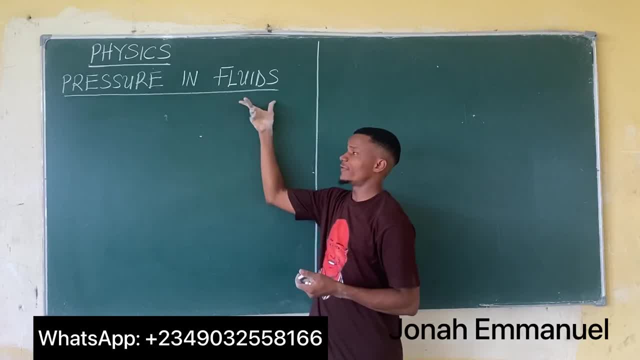 Alright, We'll look at this. What did we do? We took the solidほど to the width of the solidile, Chopped off again into two parts, So it's called a solid. So our goal for this question now is to get all the time in the Moolder scheme to$0.20.. to important, So if 3 is given. 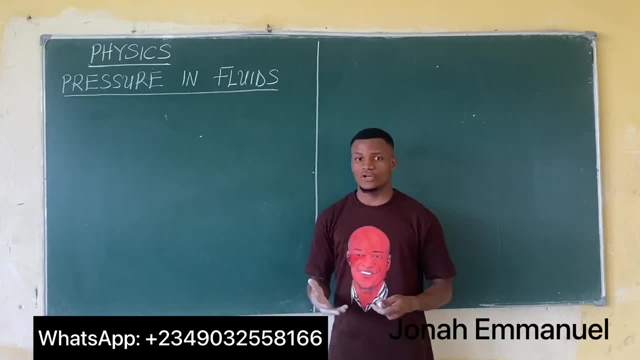 out here.0.5X equals to yard square. each time From that pun. the second step code here is to write down f cost between two hours. So what this will do isfrangel 0.5X equals to $0.3.. So the third step code here for this question now is: I'm not going to75. note up all. six feet here. I'm going to put at the m.1 NEXT, But let's leave some starts. All right, Would this help? OK, good, Ok, In god's way, though I may be able to do this. What is it? my team? look at the next. 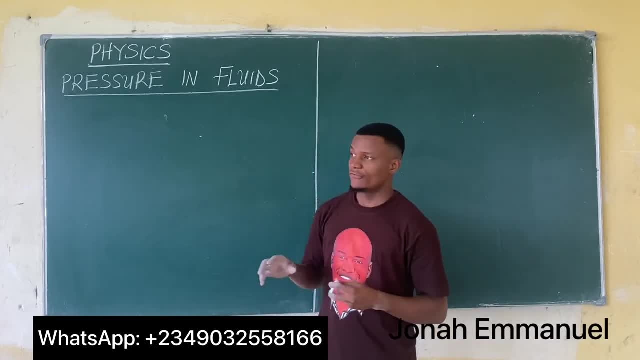 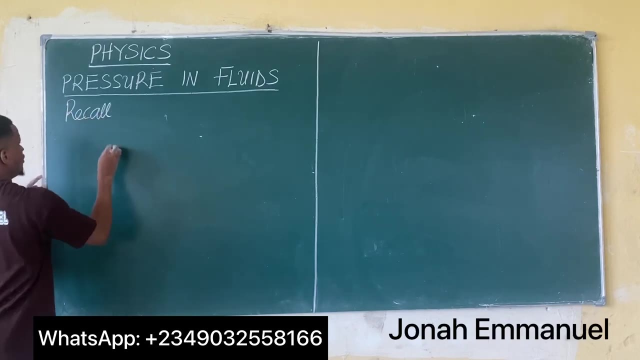 pressure for liquids and gases. Now here is what you should note: For pressure, liquids and gases, we have a different formula for measuring that, So let's try to derive the formula. First of all, let's recall what we know, Recall what we know, Recall that we. 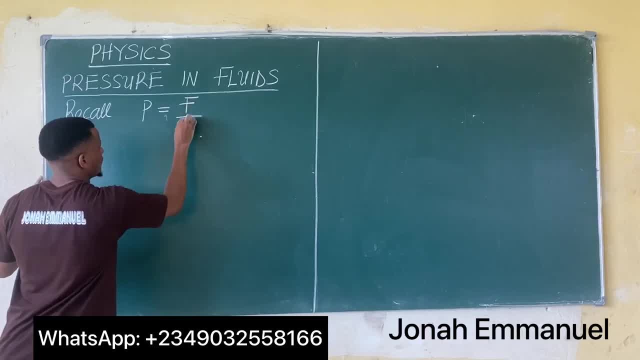 said, pressure is equal to force all over area, as we discussed. But we know that force is equal to mass times gravity. Let me call this my first equation. Call this the second equation. So force is equal to mass times gravity. If I put two, put equation, two into equation. 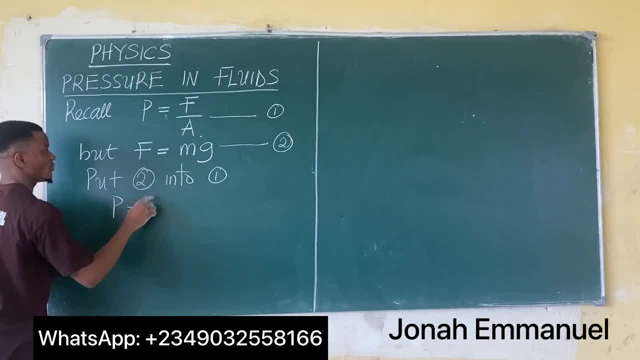 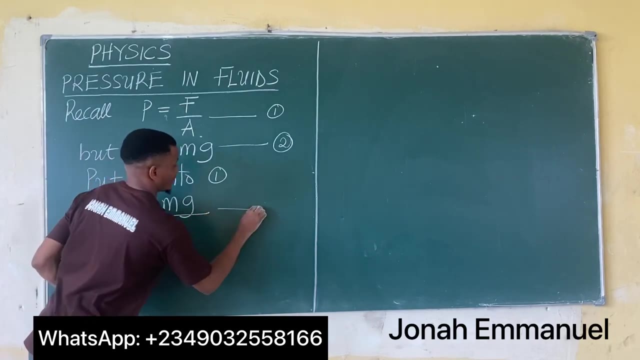 one. what do I have? I have that pressure is equal to force. Force is mass times gravity, So it becomes mass times gravity all over water area. So I've replaced force by what? mass and gravity. so I have this. you can call this equation three. let's recall something about. 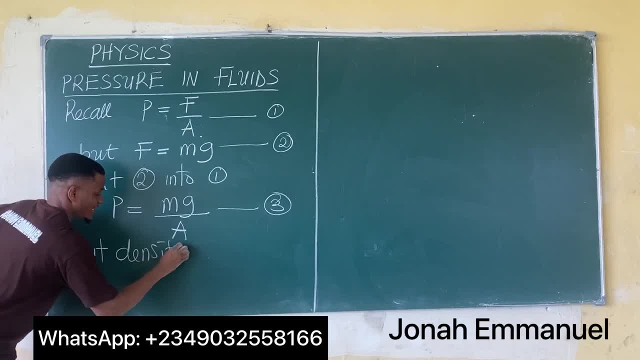 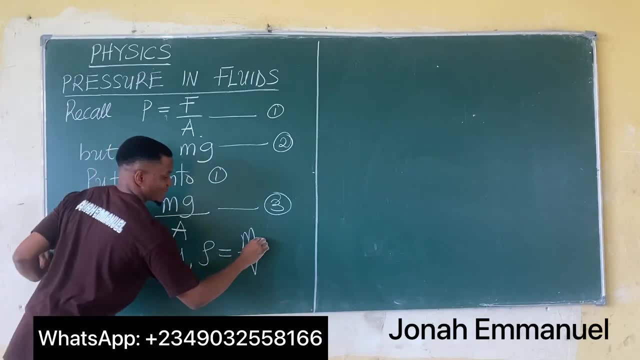 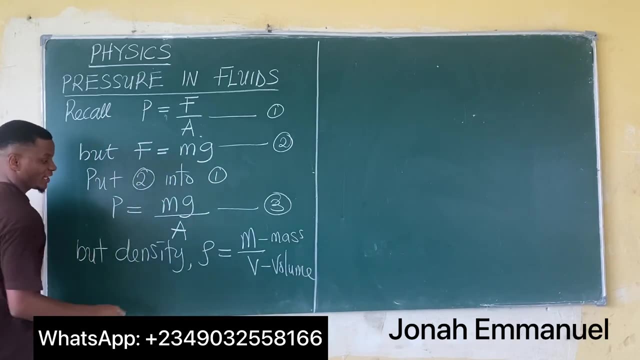 density. but density, we say density, rho is equal to water. mass all over volume, this is mass, this is volume, this is density. if I make mass something from the formula here, this is all over one, it becomes mass times one. it means that mass is equal to density. times volume gives you density. 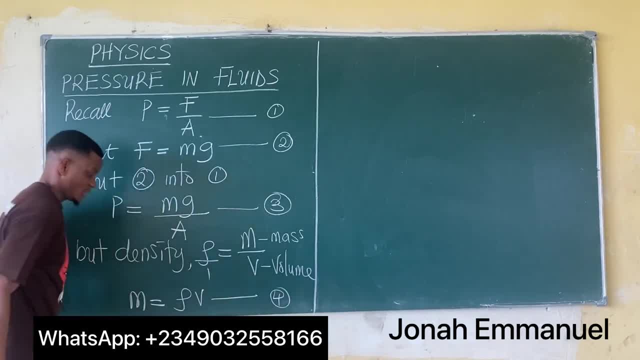 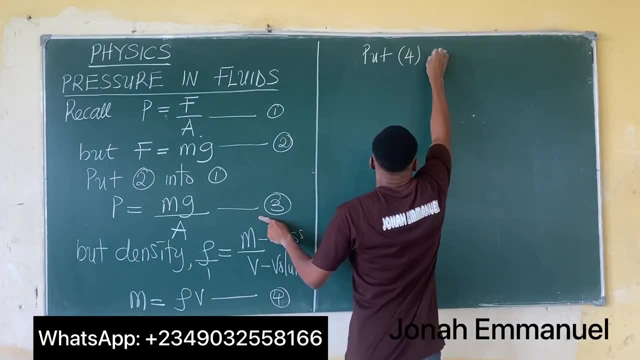 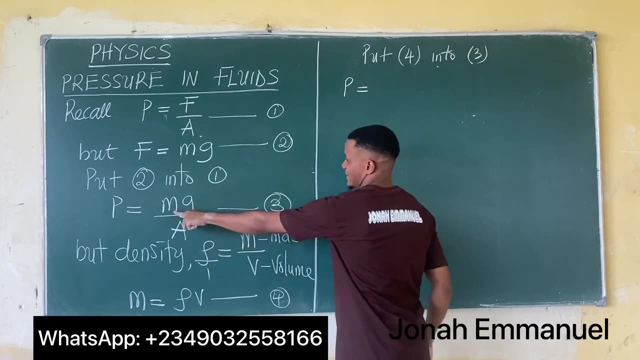 volume. call this equation four. if I put four into three, if I put equation four into equation three, it means that pressure p is equal to mass. in place of mass I'll put the value of what? density and volume. so density times volume of ice. here it becomes density times volume. of course, times this one here. 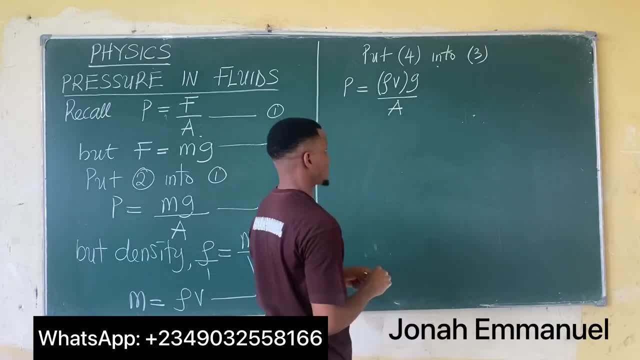 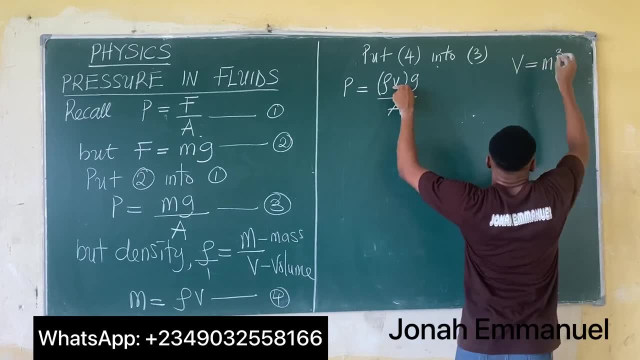 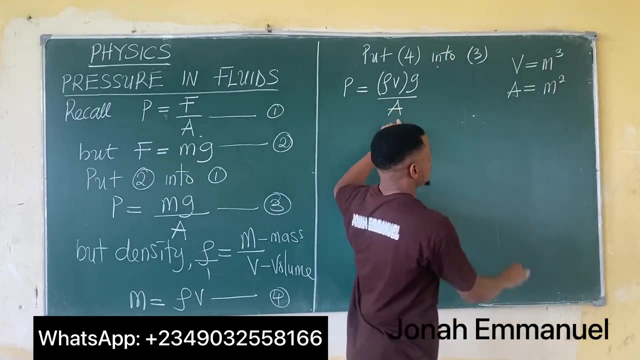 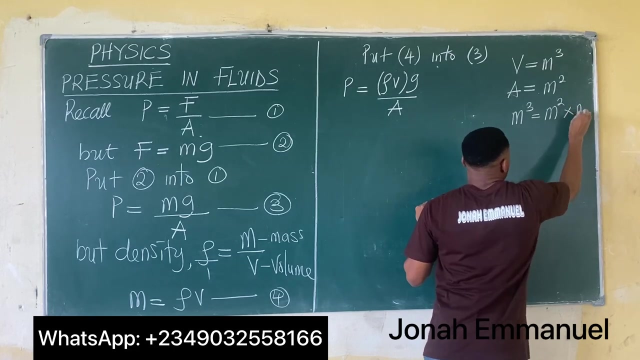 gravity all over area so I have this this is volume volume is measured in meter cube a is area measured in meter square I know fully well from my job in mathematics that meter cube is equal to � m square times das so it means that bounding which is me touch what is equal to p-sq which is area times advantage 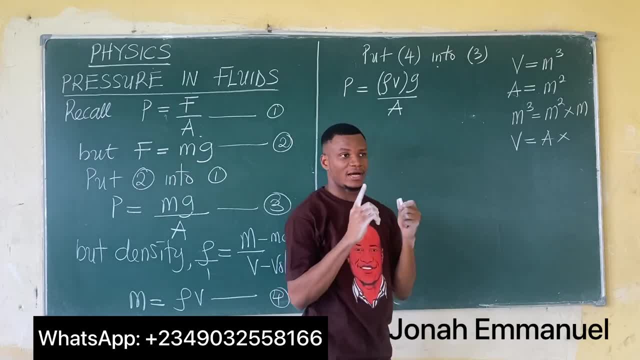 in this aspect of flu. we're taking a horizontal length. that becomes a height, becomes area. that is height means volume is equal to area and height. hia means height. all right, so hte objet, 님 Christguard, are equal to area and height, Then hia is equal to hight. 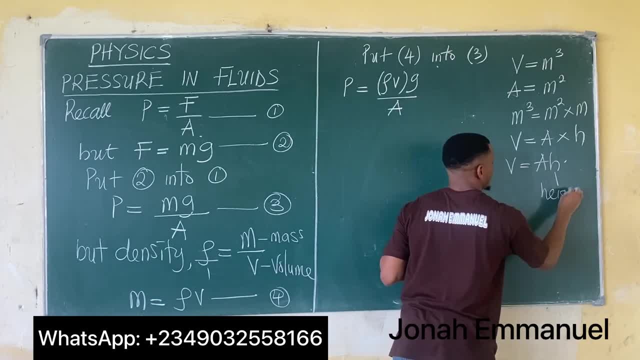 hia means height, all right. so hia equals creator being greater than height. this is where you can actually. you can actually calculate a when you take that and you actually calculate a value. so the uh value is equal to Pq weight multiplied by h height. I mean it means that Gold. 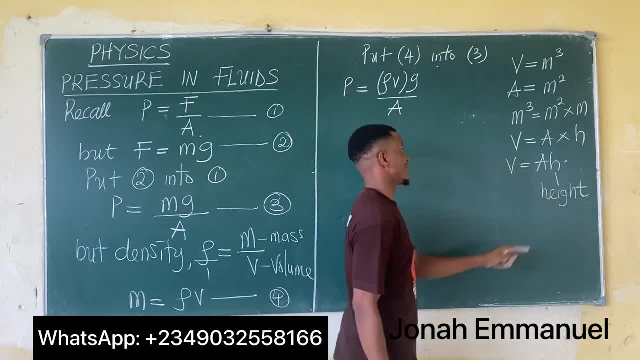 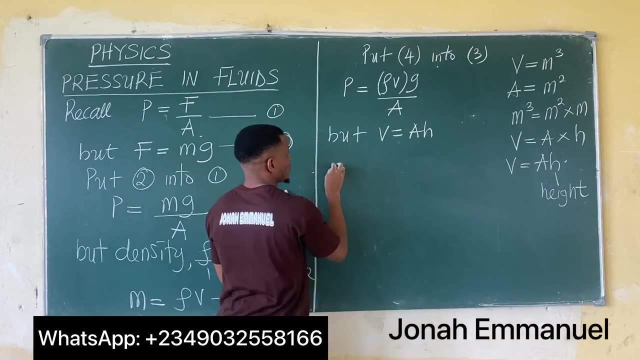 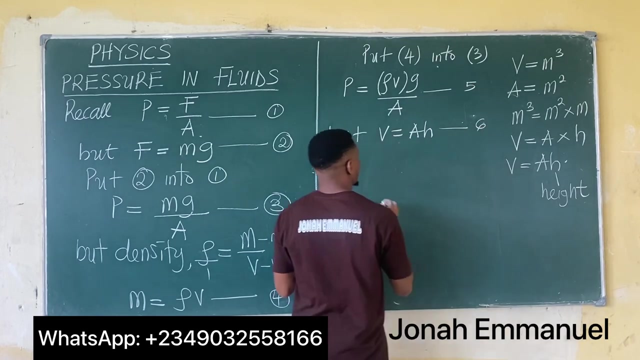 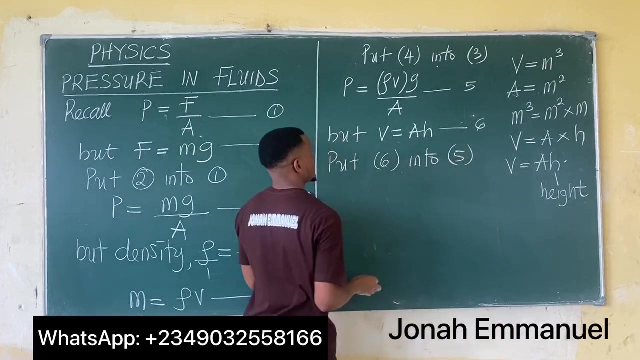 h means height, So volume is equal to area times height. So what Volume is equal to area times height? I've explained why. So meter squared times height Meter gives you meter cubed volume. Alright, if I put this here, it means that pressure. let me call this. what? Call this 5, call this 6.. Alright, if I put equation 6 into 5, what do I get? 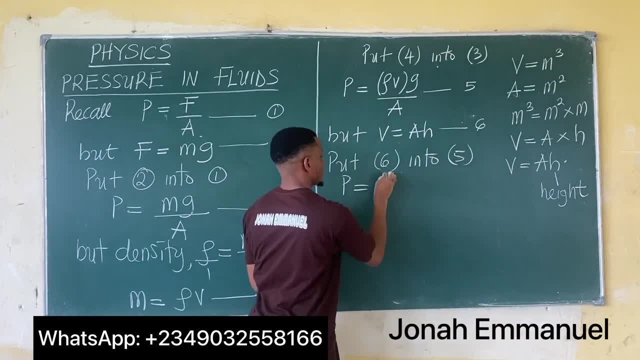 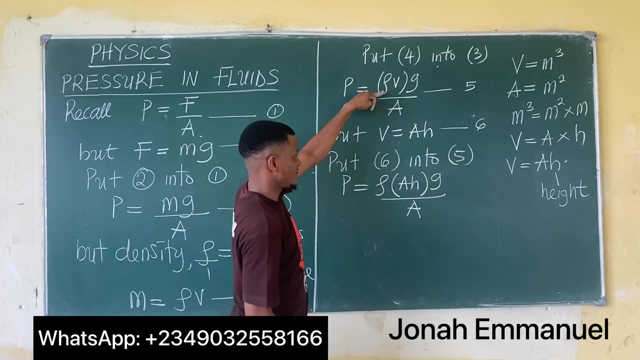 Pressure is equal to density. this times volume Volume is area times height. So area times height times gravity, this all the way. So area: nothing has changed. I only replaced volume. So density is here Volume. I replaced it by product of area times height times gravity. That's it, So I have this. 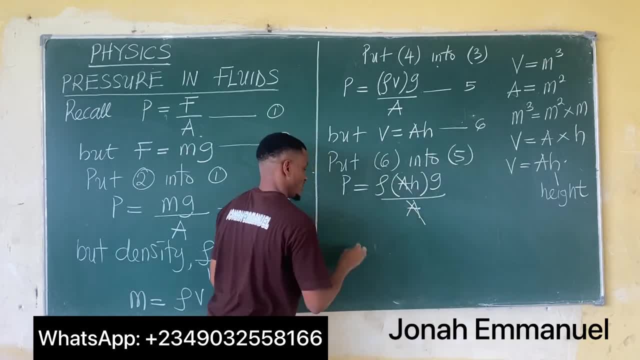 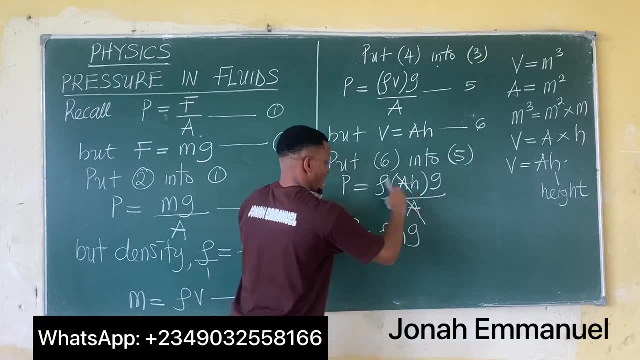 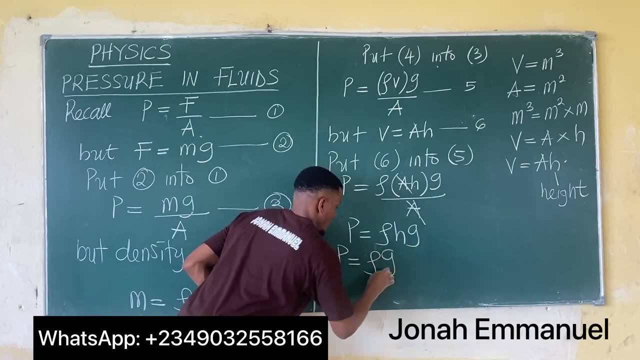 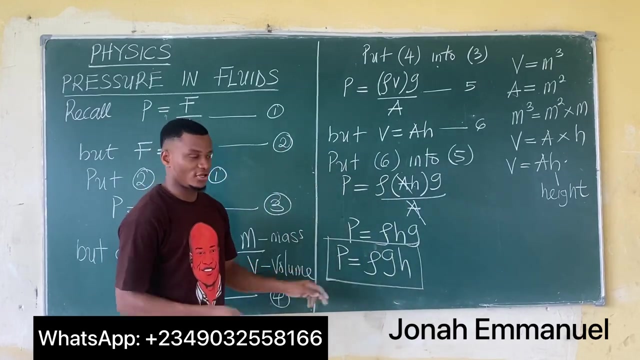 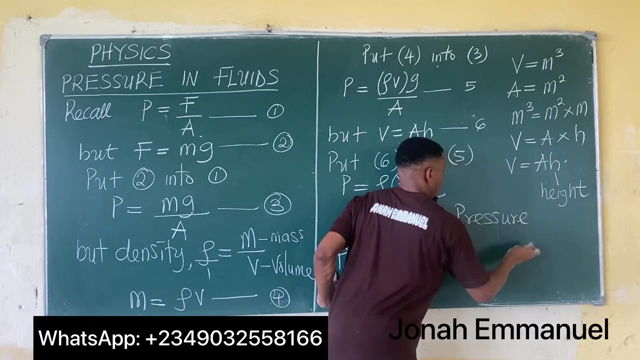 From here now, area cancels area. So pressure is equal to rho density times h times g. If I rearrange this, it means that pressure p is equal to rho density times g, Gravity Times h times. This becomes the formula for calculating pressure in fluid, Where p, we say, is pressure in Newton per meter squared. rho is equal to density in kilogram per meter cubed. 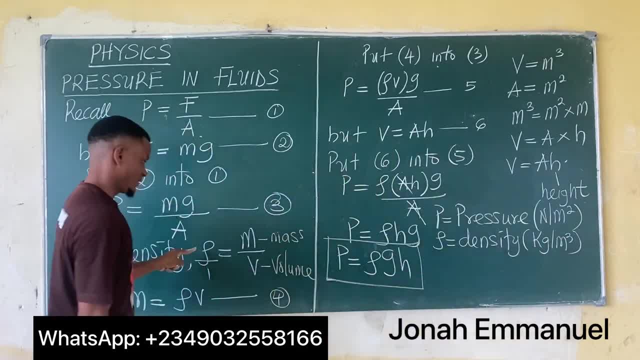 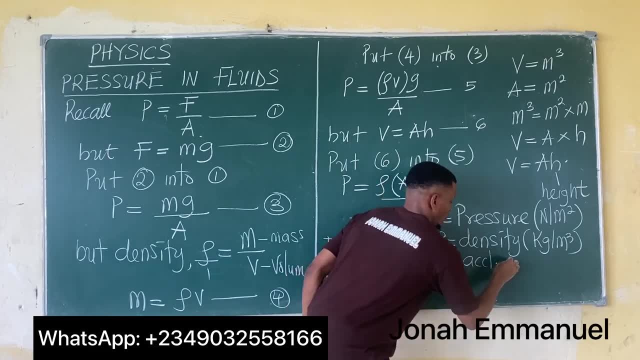 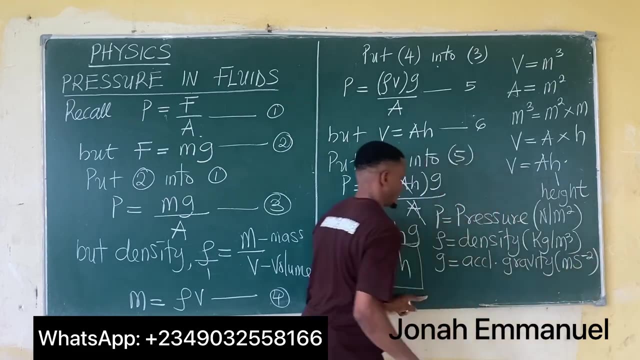 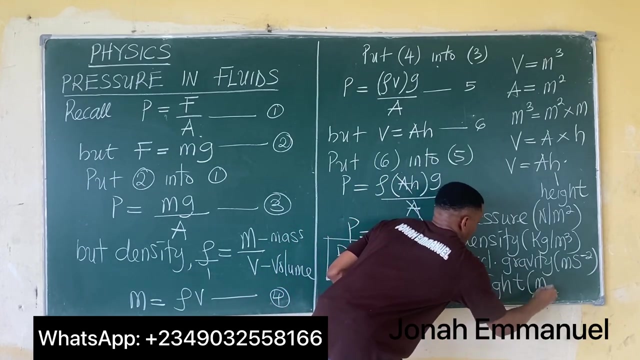 Because I'm having mass over volume, as we said there. This mass over volume g is acceleration, ACCL due to gravity. So ACCL, gravity in meter per second squared, And finding h is equal to height, Height is in meters. 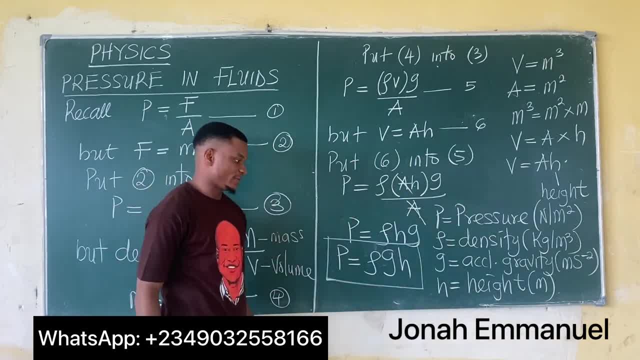 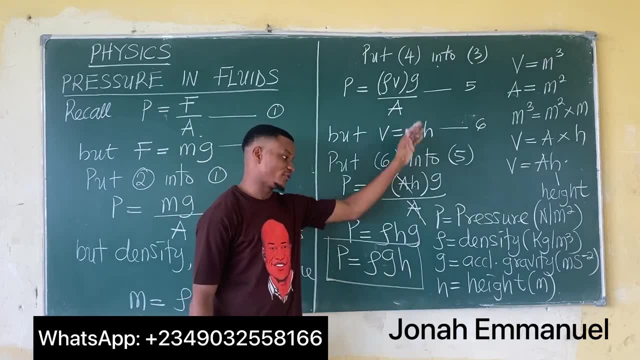 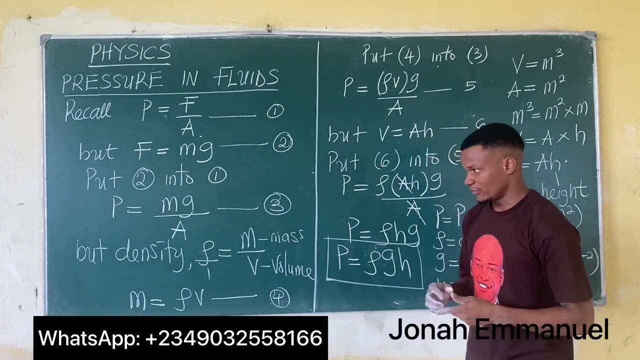 Alright, That means to calculate pressure for fluid, multiply the density of the fluid by acceleration due to gravity, By acceleration due to gravity, by the height of the fluid. So this is my formula for pressure in a fluid, whether in liquid or in gas. 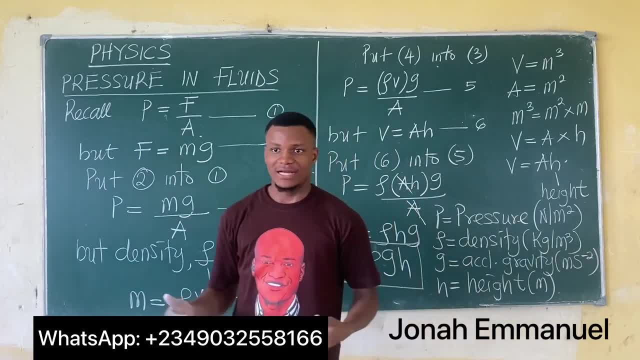 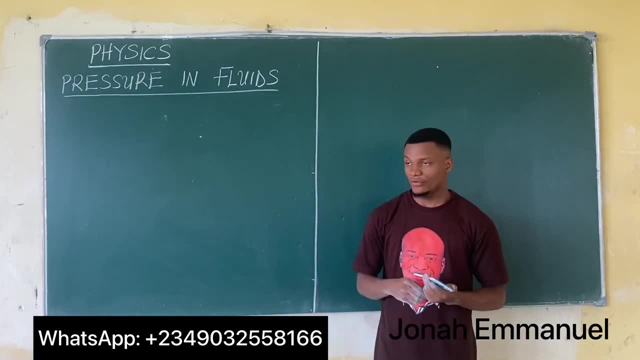 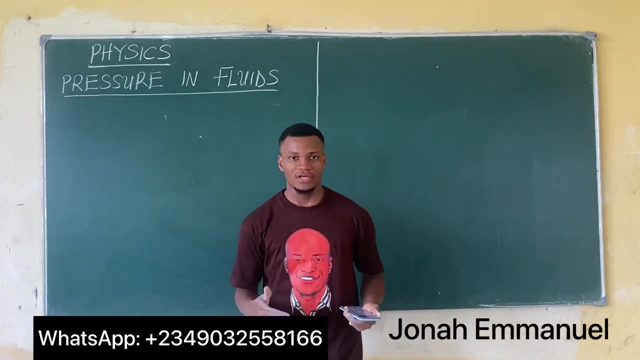 We'll take some sample problem we'll solve together and then we'll look at some jammed past questions on pressure. Alright, so we'll take some questions on pressure in fluids and so on. By the way, we just derived the formula for pressure in fluids as P equal to rho gh. 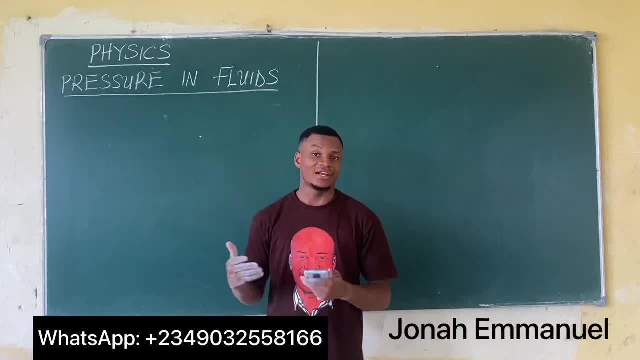 Now it doesn't necessarily mean you have to go and start cramming the derivation. I would have just given you the formula, but I thought it wise to do the derivation first, So you don't start asking how, how, how. But if it's too complex you can just forego the derivation. 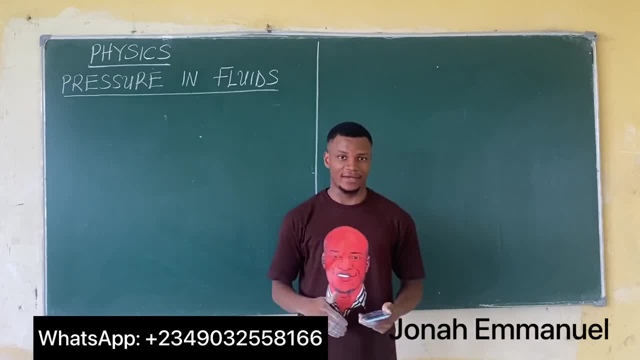 But always remember that pressure is equal to force over area In terms of solid, and pressure is equal to density times gravity times height In terms of fluids, that's liquids and gases. Alright, having said that, let's take some examples. 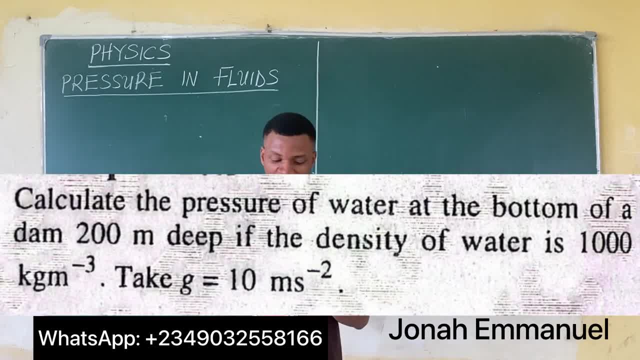 So let's look at this example. Example 1 says: calculate the pressure of water at the bottom of a dam 200 meters deep. If the density of water is 1000 kilogram the meter cube, take gravity to be equal to 10 meter per second squared. 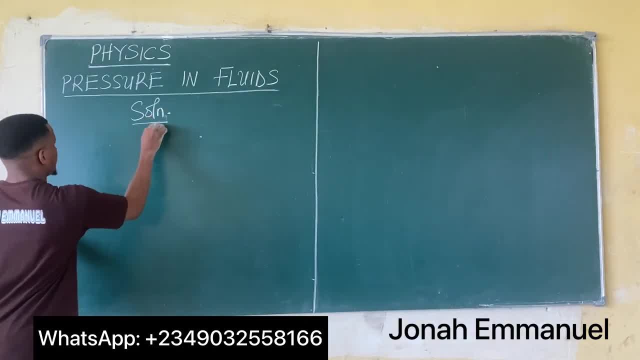 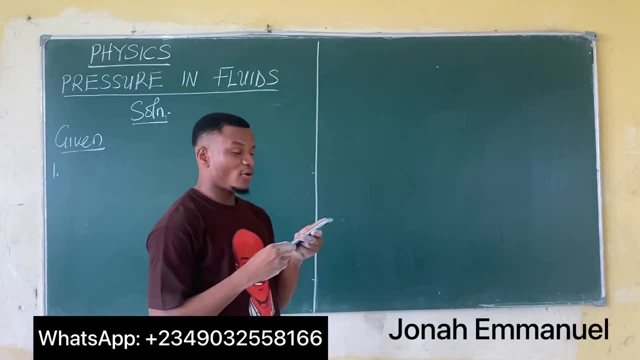 Alright, So let's look at this solution. We start giving parameter number 1.. It says: calculate the pressure of water at the bottom of a dam 200 meters deep, And that's what it says when it comes to pressure in fluids. Look at the height. 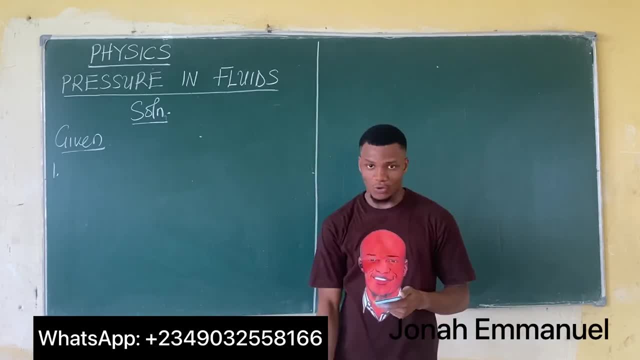 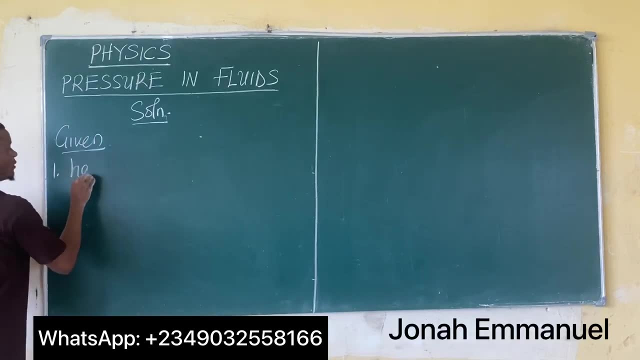 So that means the height from the height of the dam below or downwards. What's that? 200 meters? That's what it says. Deep, Alright. So number 1. I'm giving height. Height H Is equal to 200 meters. 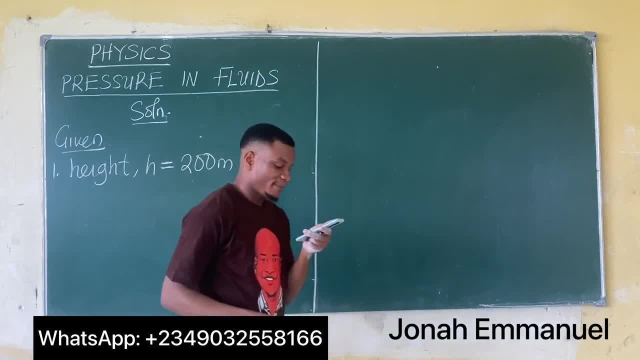 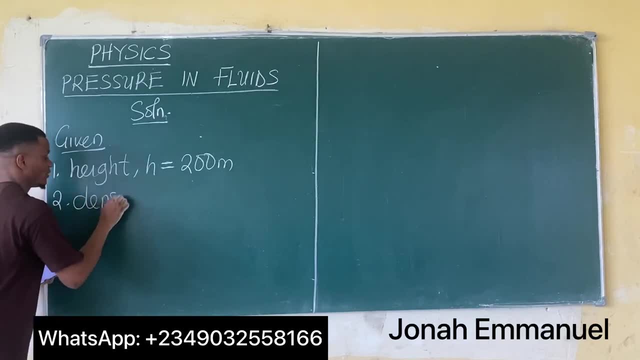 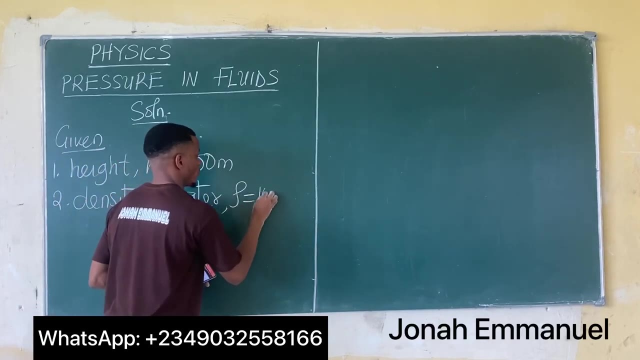 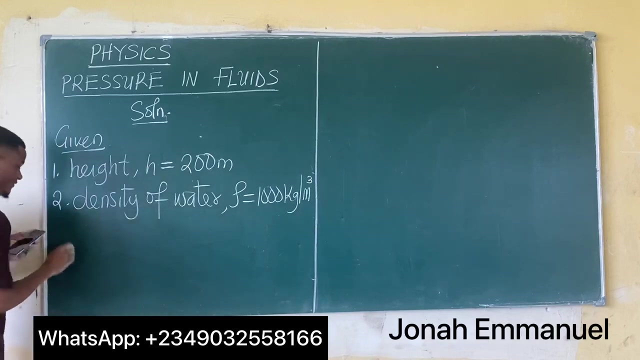 I have this What they want to say If the density of water is 1000.2.. Density of water. Density of water. Some video room has 1000 kilogram per meter cube And they said Gravity G. 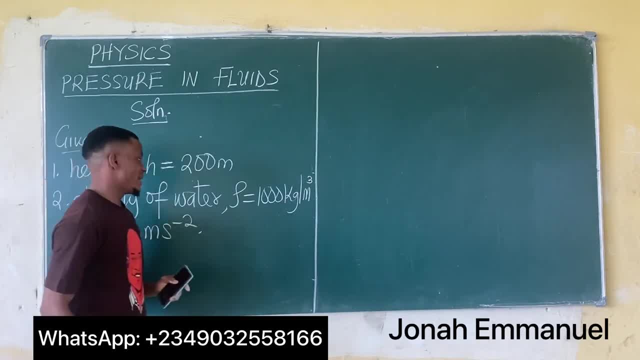 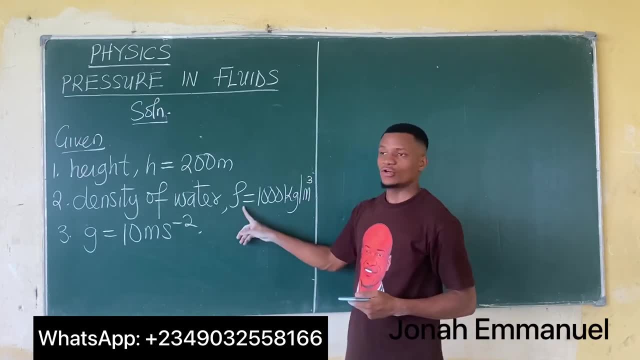 As being 10 meter per second squared. They have to find the pressure. Now let me say something Straight up. The density of water is always a constant And the value is 1000 kilogram per meter cube Or 1 gram per cm cube. 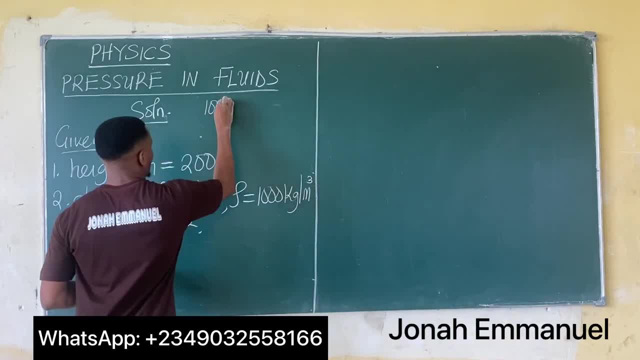 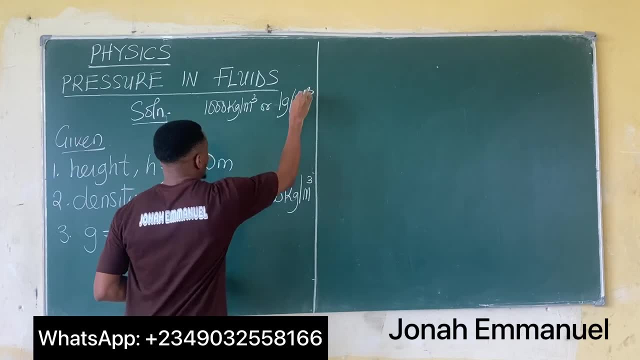 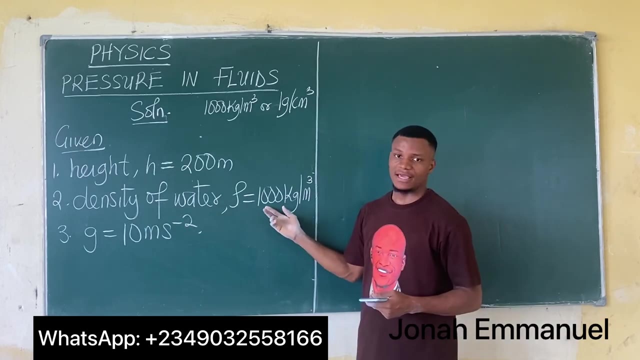 Alright, Don't forget this: 1000 kilogram per meter cube, Or 1 gram per cm cube. So, in other words, You would Not be giving the value of density of water. That would be Anything aside this. So it's always 1000.. 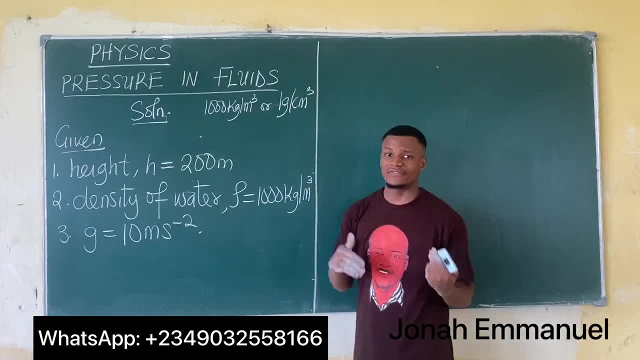 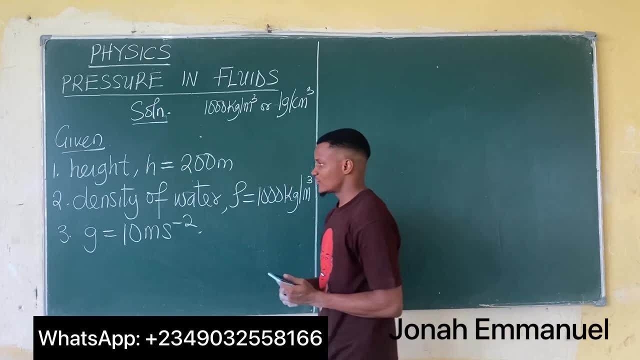 So that means, Whether you're giving density of water Or you're not giving, So fast is water. The density is always water 1000.. So please always notice this way. Alright, So that's so. We have that pressure. 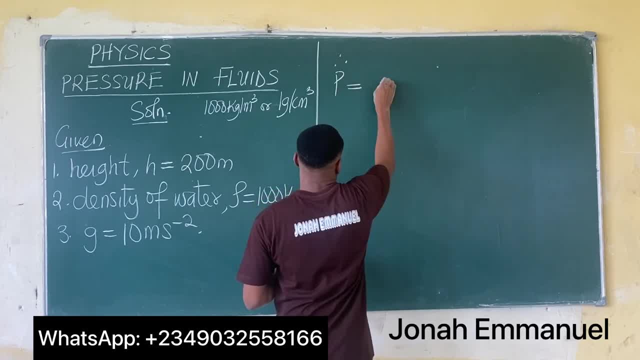 So therefore, The pressure of P Is equal to Rho, Times G, Times H, And that's equal to Density of water: 1000.. Times, gravity: 10. Times The dam Is 200.. Alright, 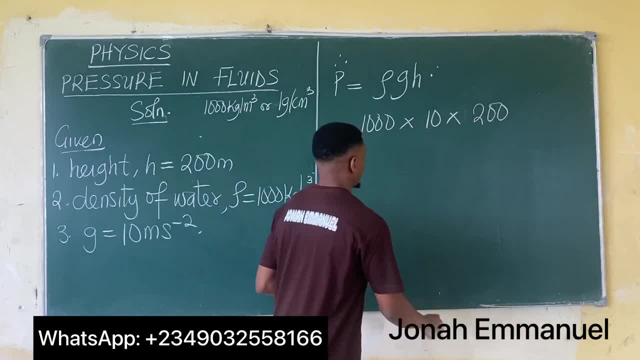 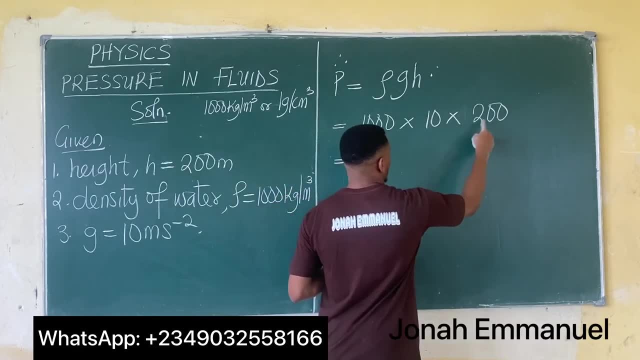 So let's get this done. This is equal to: If I multiply all of this, And it comes to 2.. Simply count number of zeros: 1., 2., 3., 4., 5., 6. So 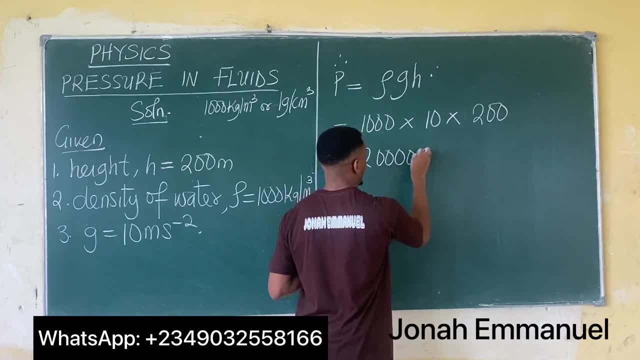 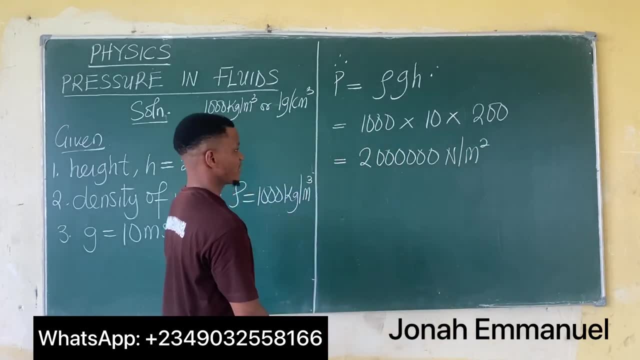 1., 2., 3., 4., 5., 6. Pressure is measured in Newton Per Meter Square. So this is my answer. Perhaps I should do some compression From here. I'm having 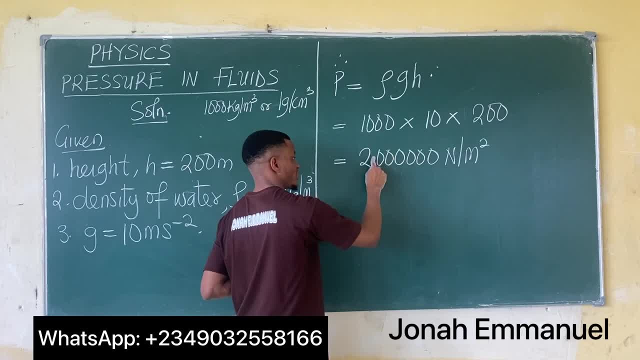 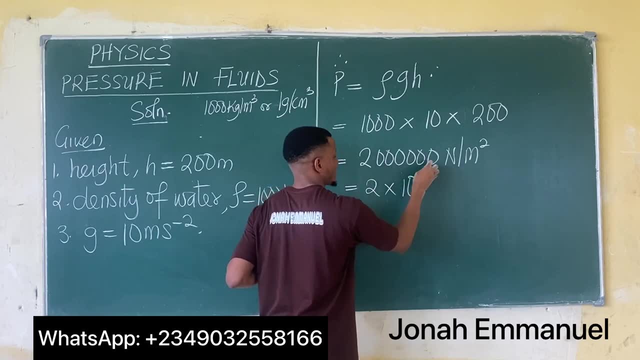 1., 2. 3. That's kilo. 1. 2. 3. That's Mega. So that's equal to 2 times 10 to the power 1. 2. 3.. 4., 5., 6., 7., 6., 7., 8., 9., 10., 11., 12., 13., 14., 15., 16., 17. 18.. 19., 20., 21., 22., 23., 24., 25., 26., 27., 28., 29., 30., 31., 32., 33., 34., 35.. 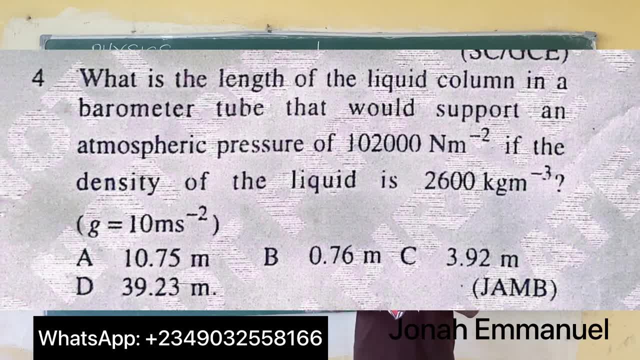 36., 37., 38., 39., 40., 41., 42., 43., 44., 45., 46., 47., 48., 49., 50., 51., 52.. 53., 54., 55., 56., 57., 58., 59., 60., 61., 62., 63., 63., 64., 65., 66., 67., 68.. 69., 70., 71., 72., 72., 73., 73., 74., 74., 75., 76., 76., 77., 78., 78., 79., 79.. 80., 80., 81., 82., 83., 82., 83., 84., 85., 86., 87., 88., 89., 90., 91., 92., 92.. 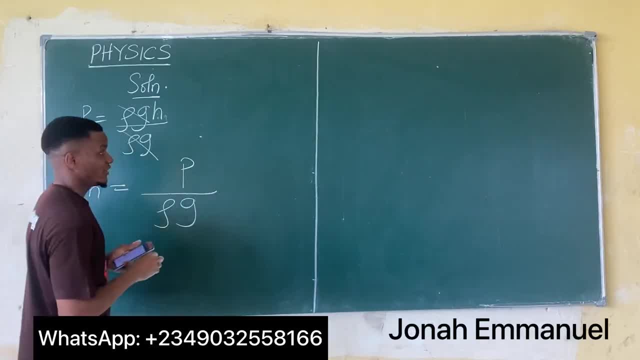 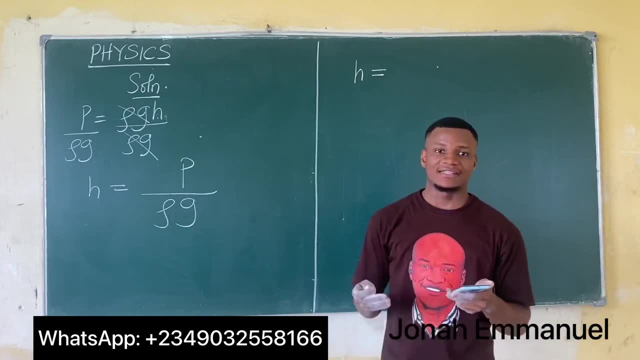 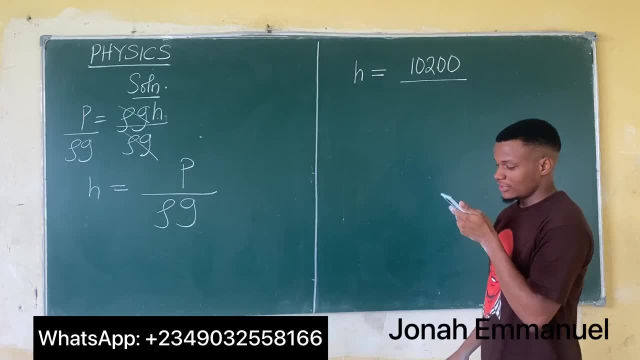 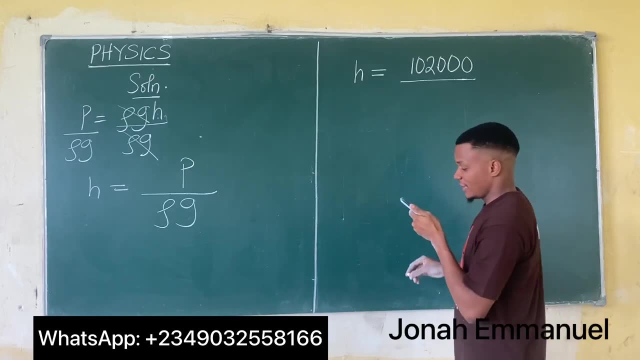 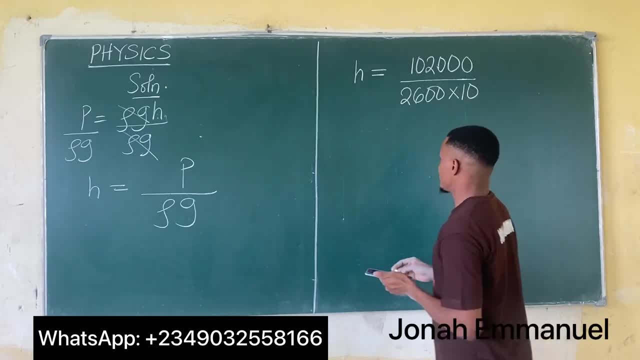 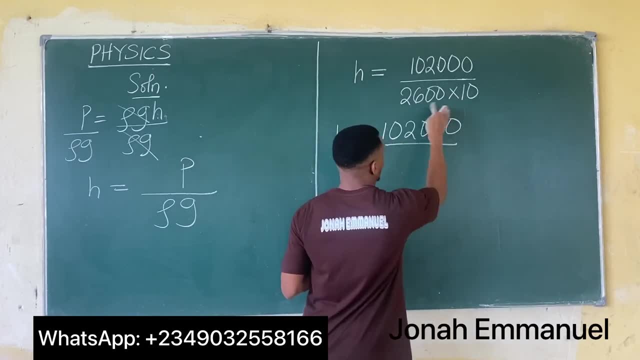 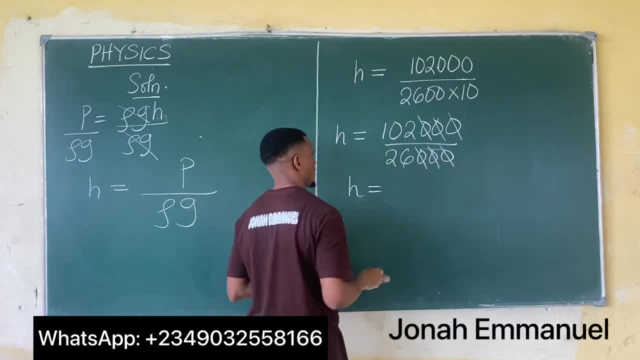 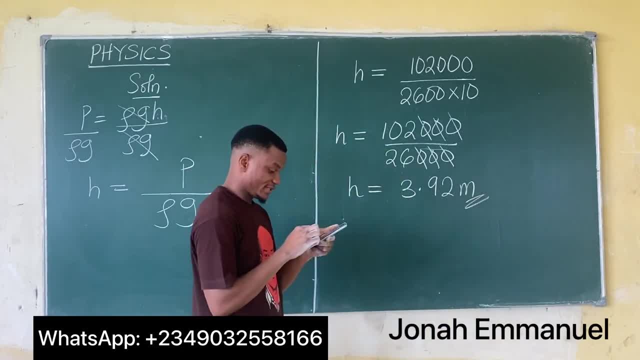 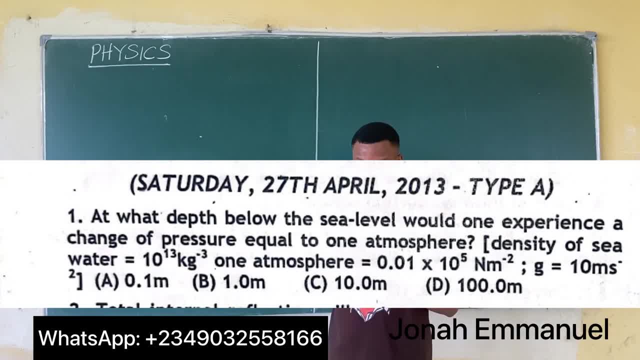 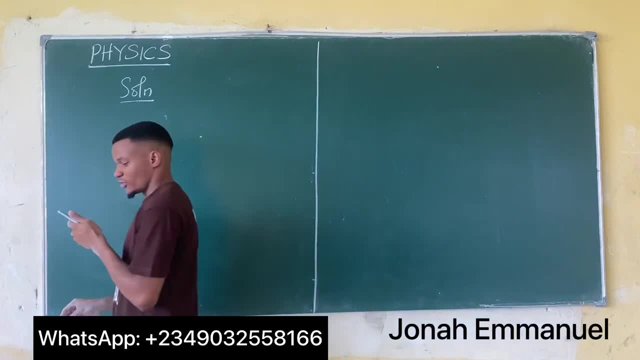 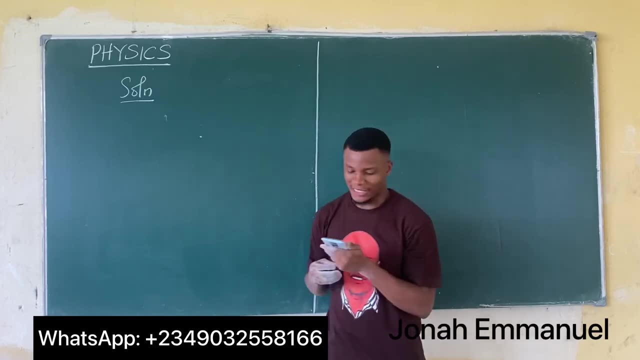 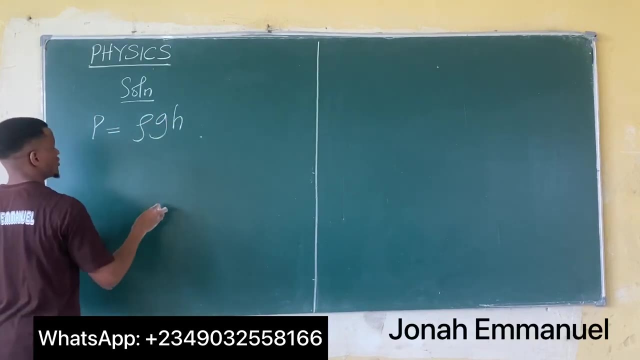 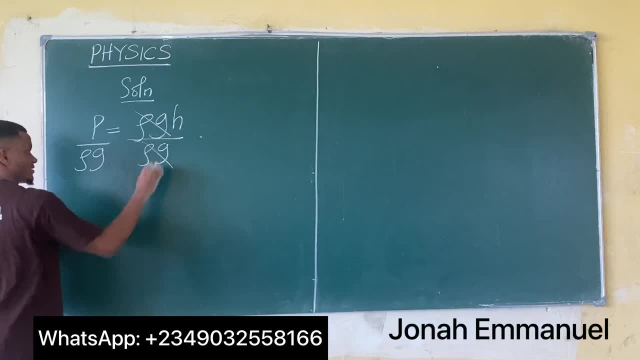 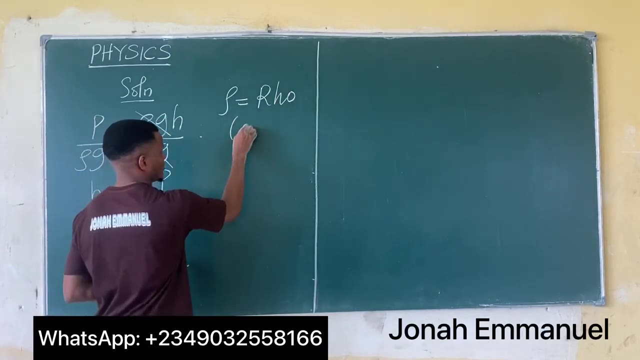 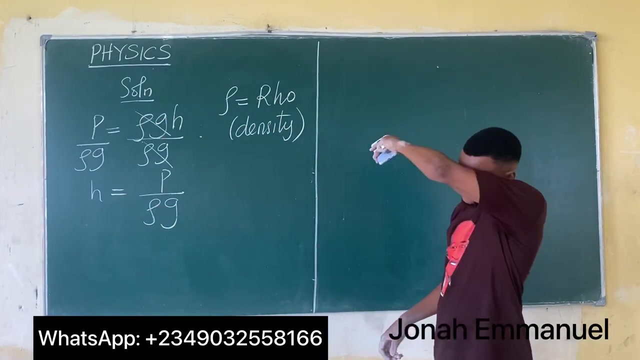 divide here by rho g is cancel this. all right, so h is equal to p. all over density and gravity. by the way, this is called rho. it's a big symbol of rho. it's pronounced rho, and represents what? density? just for you guys, it's called rho and represents density, all right, so so this is equal. 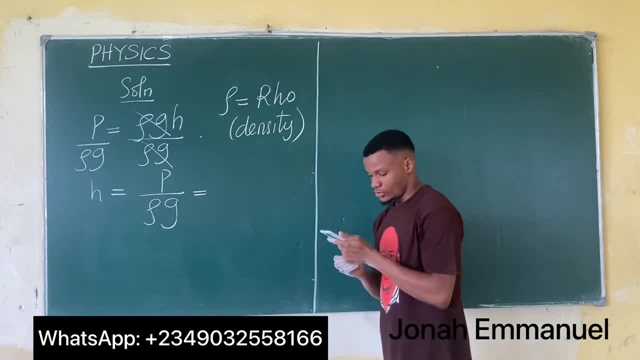 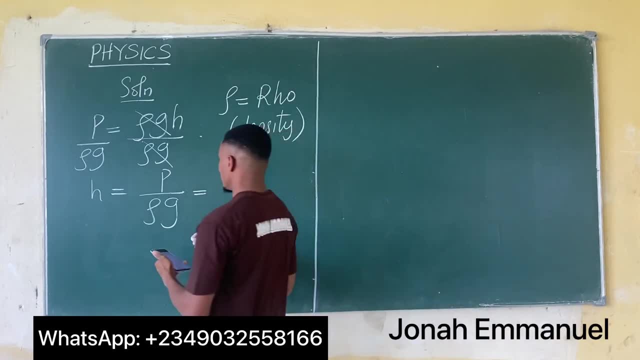 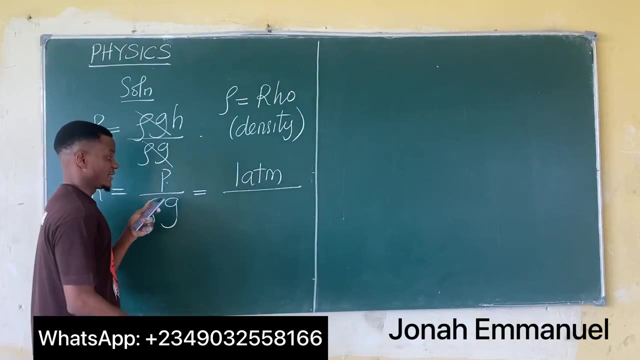 to you say at what depth would you say below the sea level? we would want to experience a pressure equal to one atmosphere. you said this pressure should be one atmosphere all over. you gave it density of the sea water as 10 to the power is that 13? 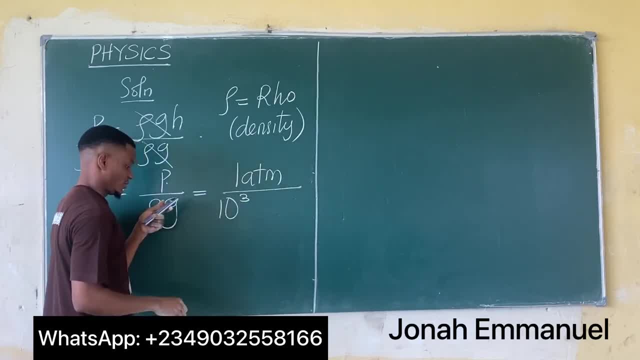 that should be 1 to 3, not 13, so 3 times. and, of course, density of water: that should be 3, not 13, 3 times. gravity is a 10, all right, so this will now be equal to. so in this case, you're giving. 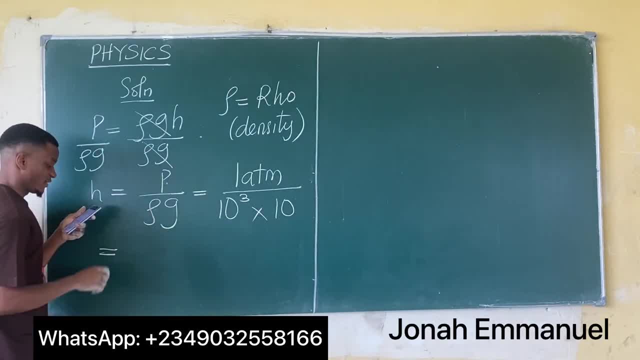 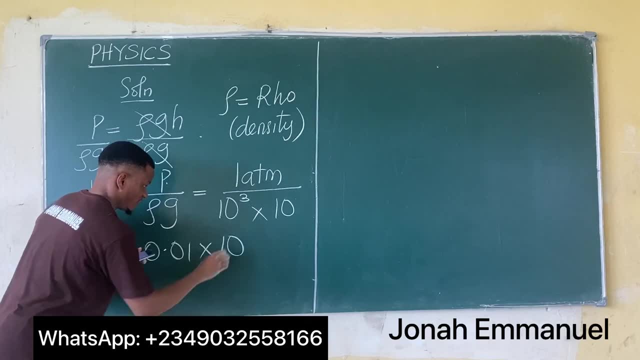 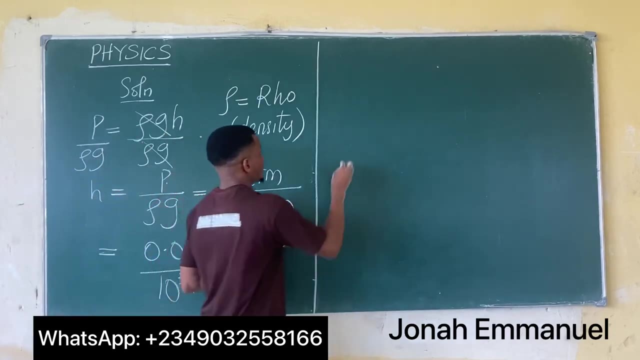 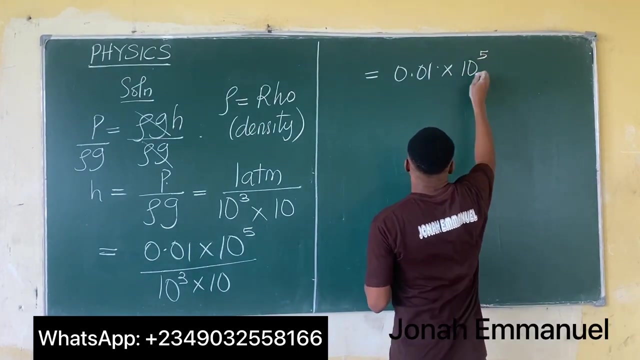 one atmosphere check. you're giving value of one atmosphere in your question, then as 0.01 times 10 to the power 5 all over, this is 10 to the power 3 times step. so this is equal to 0.01 times 10 to the power 5 all over. this 2 gives you. 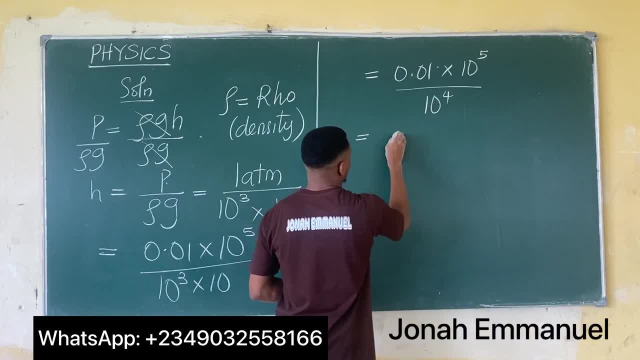 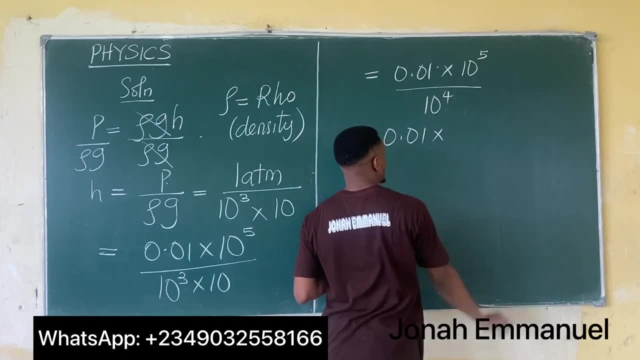 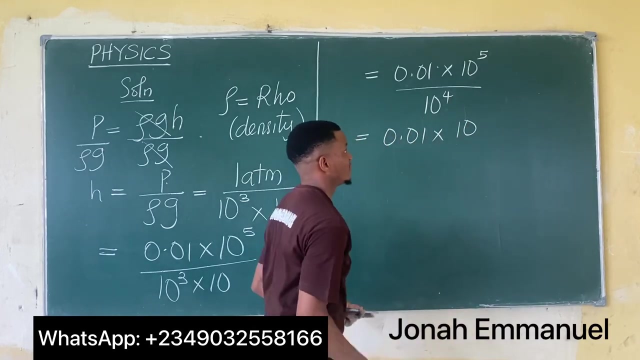 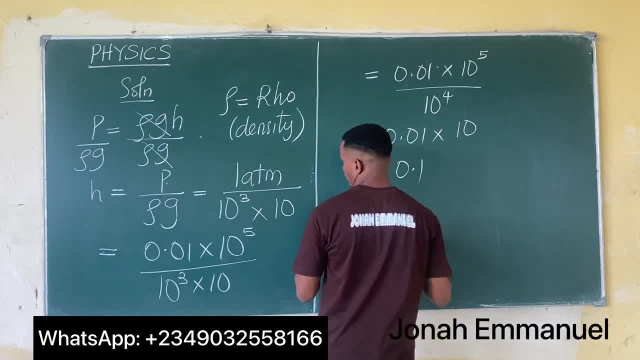 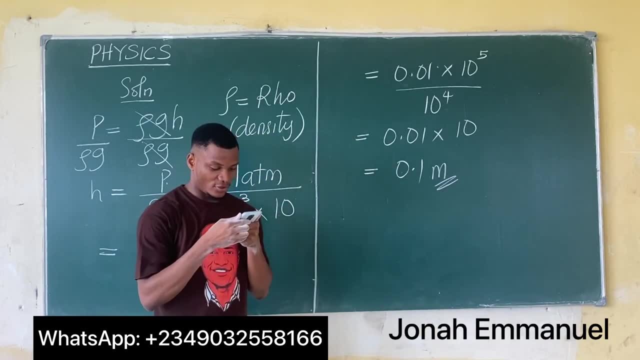 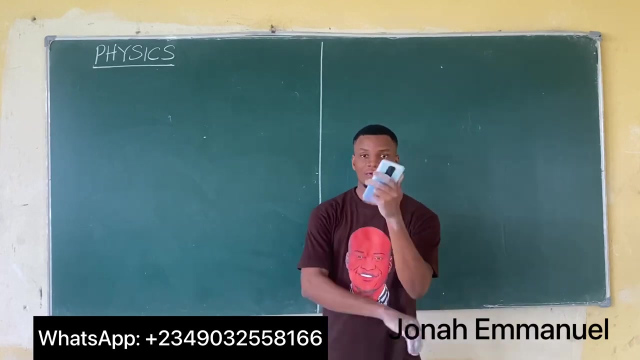 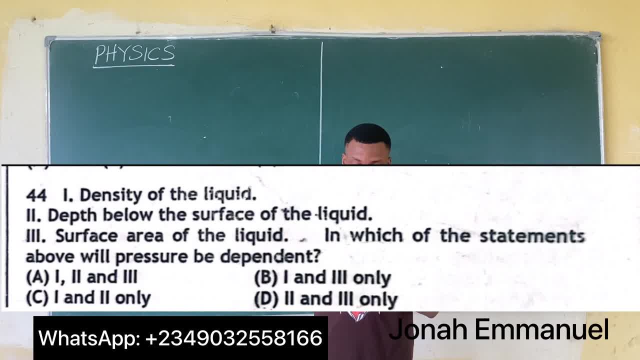 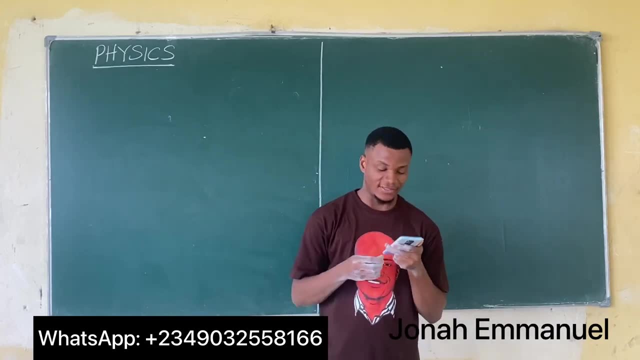 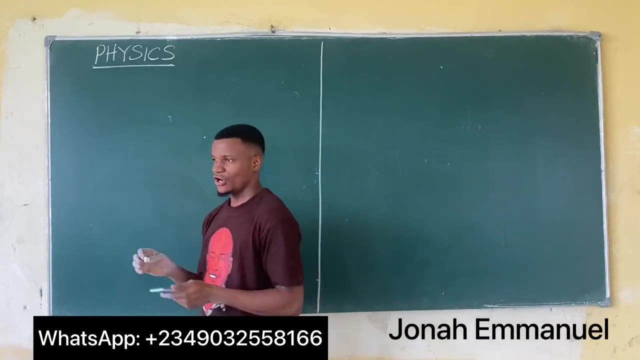 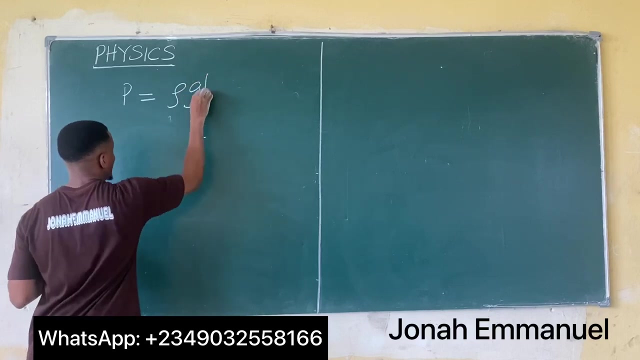 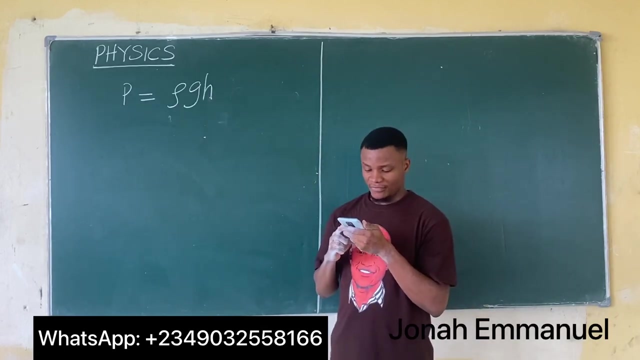 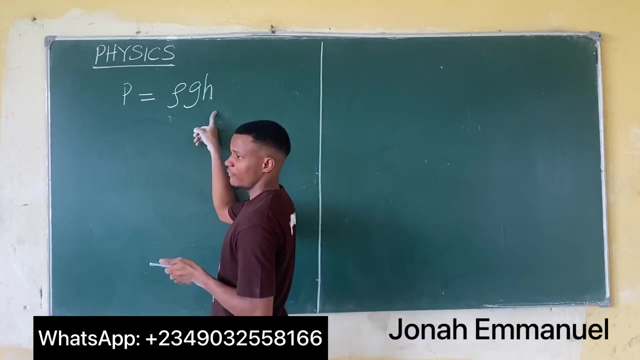 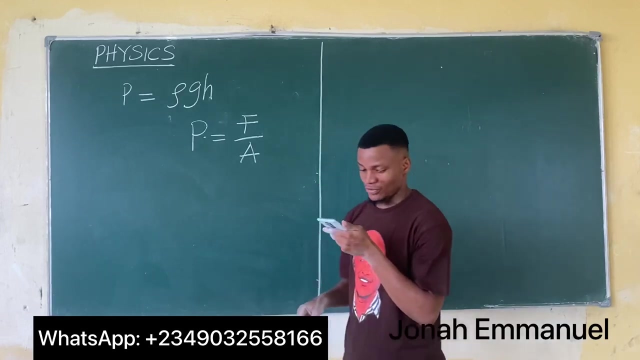 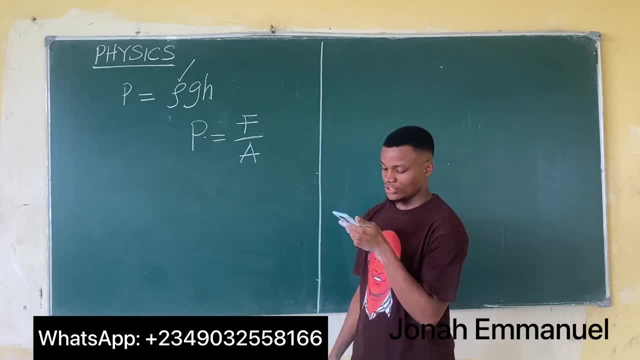 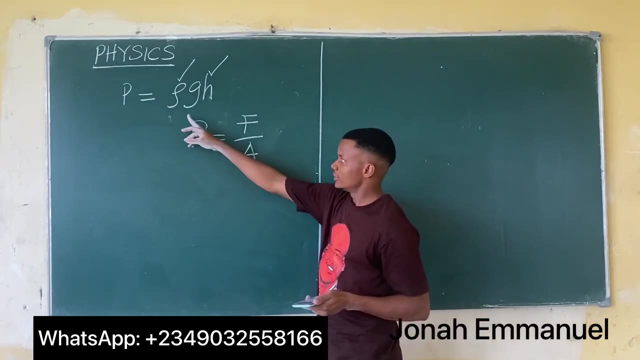 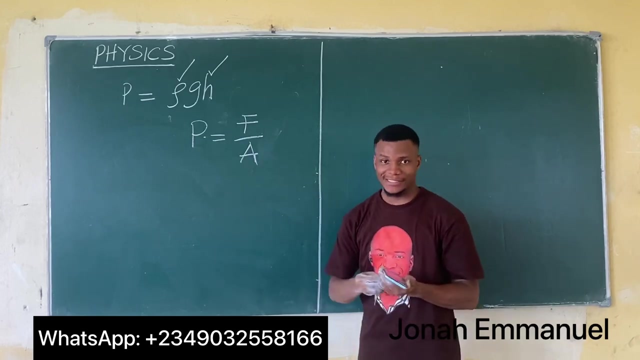 number two says depth: depth below the surface of the liquid. that's depth below the surface of the liquid or height. so it also depends on this. the next one there says surface area of the liquid. okay, so it depends on density and depth, but when it comes to area, area is for solid, so pressure. 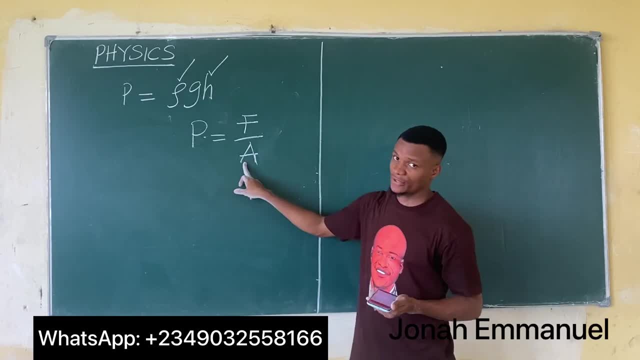 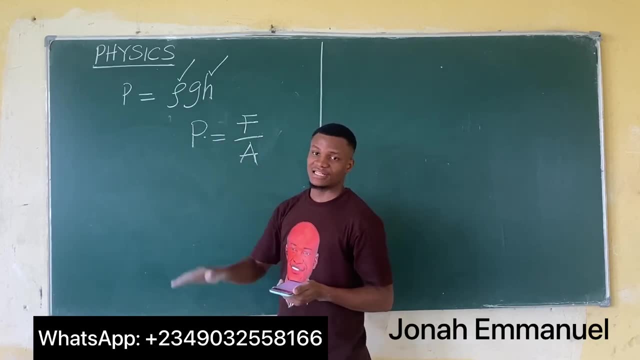 depends on the area of is solid, not a degree. so when it comes to liquid it depends on just depth, of degree and the height in which the or the depth as a liquid doesn't apply. so for pressure, area is, uh, it's not that important. so pressure does not depend on the carrier of electric. 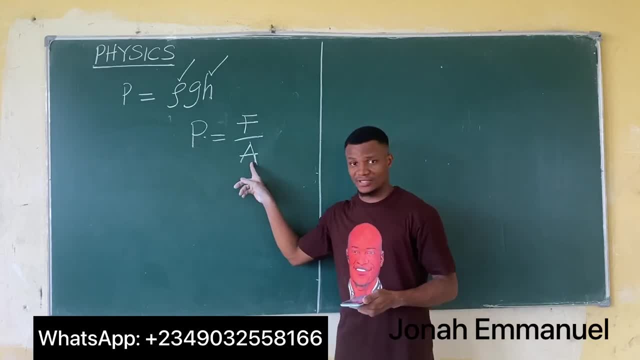 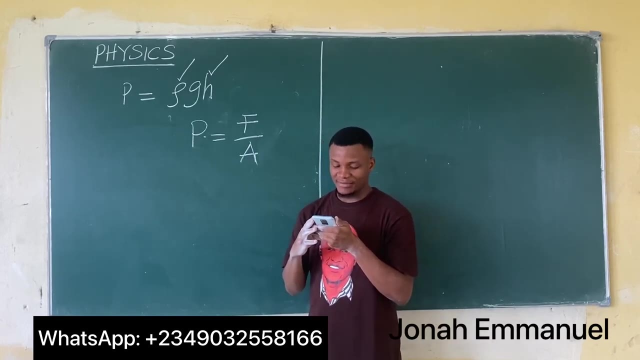 instead it depends on the area of what is solid, not liquid. so that means in this one here it is just density and depth, that's just i and ii. so the correct option then is c, which says i, density of the liquid and depth below the surface of the liquid, that's ii. so it's just i and ii only. 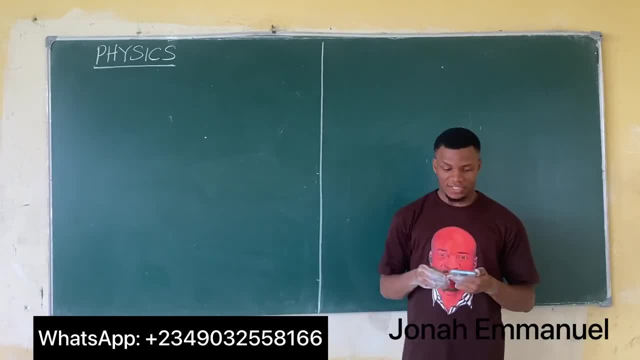 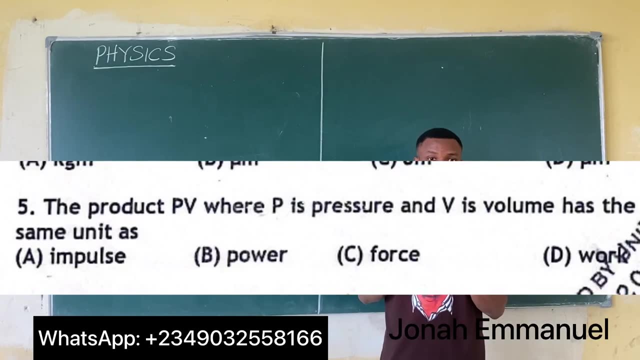 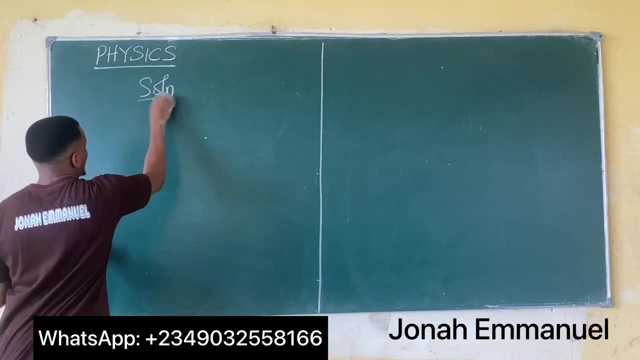 that's the correct answer. all right, so let's try this question here. this question says the product pv, where p is pressure and v is volume, has the same unit as dash and you have your options there. so solution: we are given a product of p and v. i would say p means pressure and v is volume. 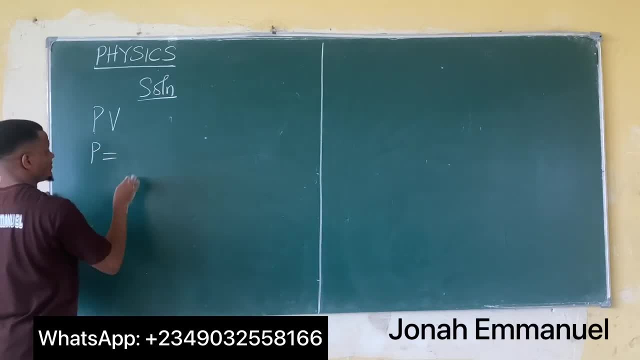 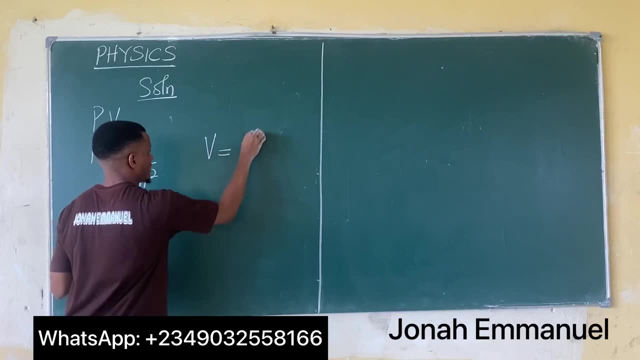 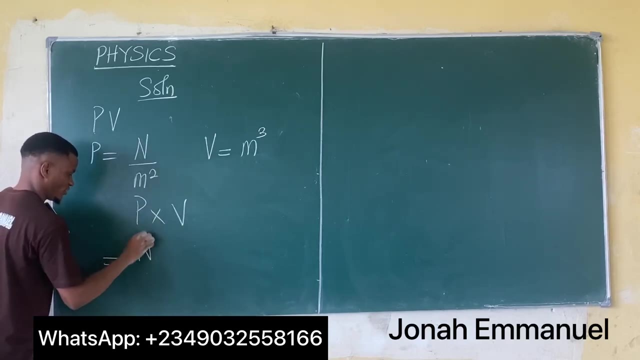 so let's get this done. p is pressure. pressure is measured in newton per meter square. that's this. v is volume. volume is measured in meter cube. so let's get the product. so p times v is equal to p is newton per meter square times v. 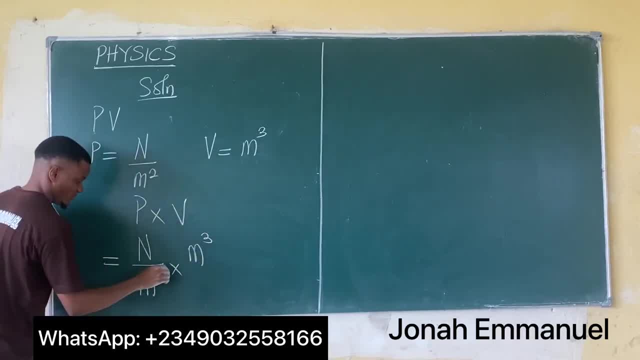 volume is meter cubed Meter squared here: 1. This cancels here: Only 1 is left. So this is 2.. This is 3.. So this cancels this. Only meter is left. If I multiply this, this is: 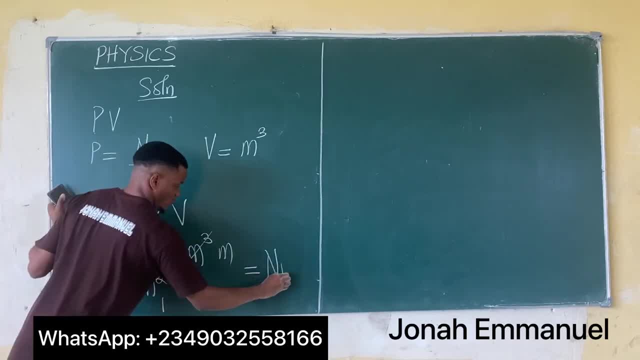 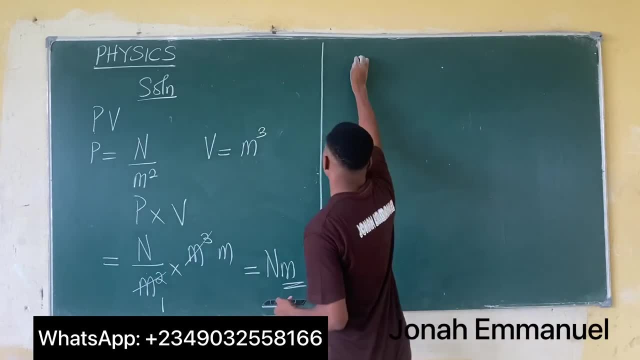 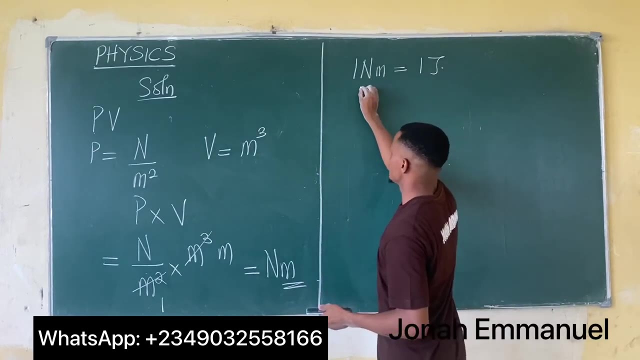 equal to newton times meter, which is newton meter? And newton meter is the same as what, then Joules? We know that 1 newton meter is equal to 1 joules. How Newton is force times meter? is what Distance? Alright. So when we talk about force times distance, what? 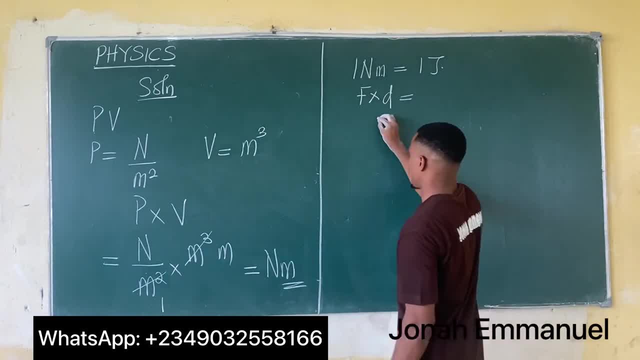 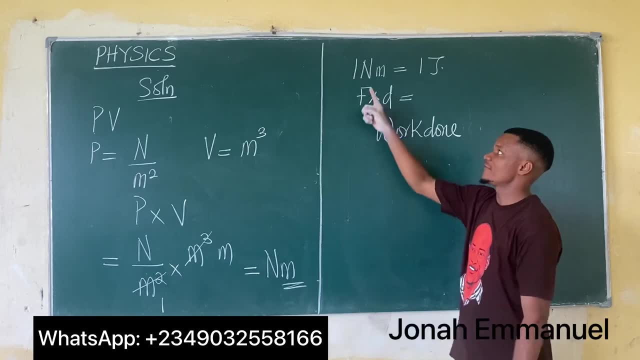 comes to mind, then Walk down. Alright, That's walk down or walk, Because it says in science, walk is said to be done when a force moves an object through a distance In the direction of that force. So hence the answer becomes walk down, which is similar. 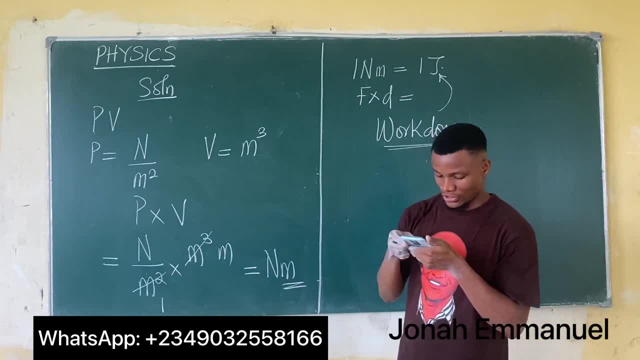 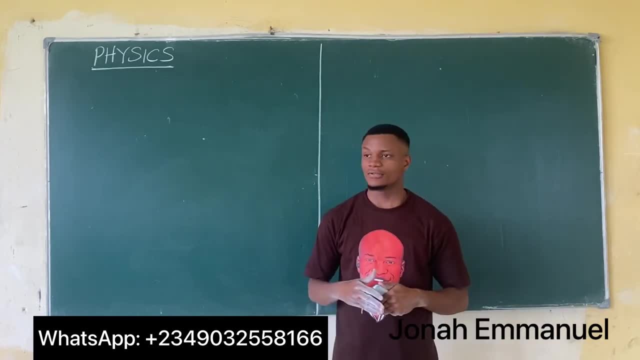 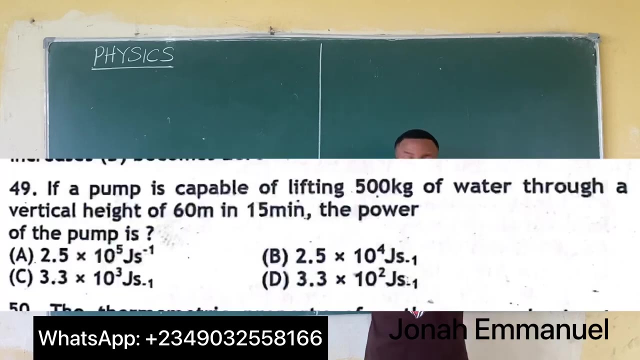 to joules. So the answer there is option D- walk. So take a final example on pressure And alright. so the question says: if a pump is capable of lifting 500 kilograms of water through a vertical line, what is the pressure? And the answer is: if a pump is capable of. 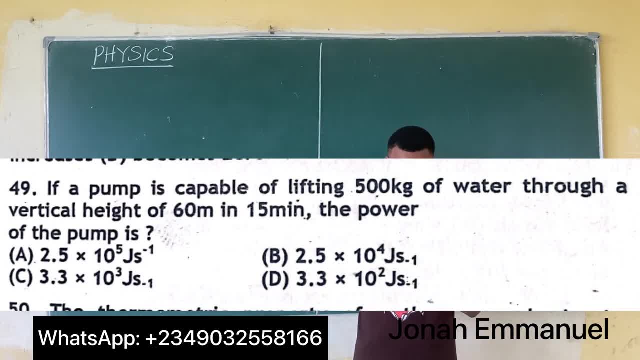 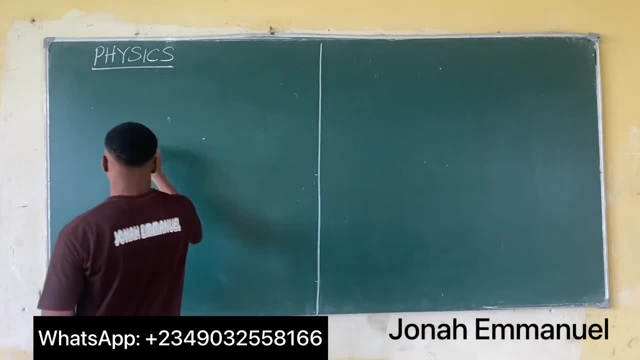 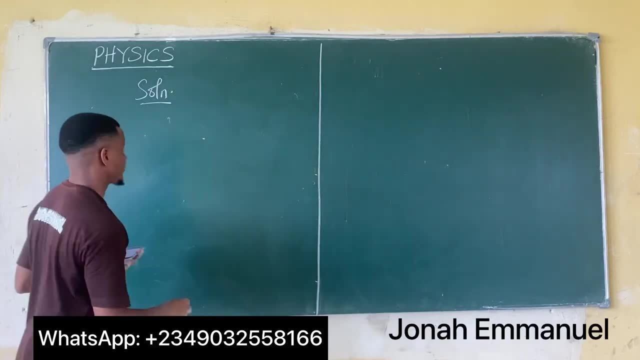 lifting 500 kilograms of water through a vertical height of 60 meters in 15 minutes. the power of the pump is so you have your options there. Alright, let's get this done. The solution- the solution that shows- is if a pump is capable of lifting 500 kilograms of water and giving 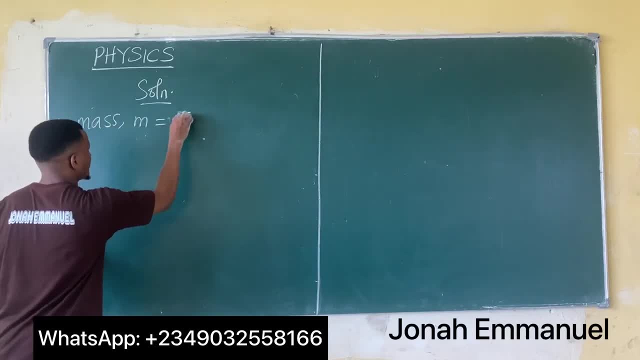 mass of pump m equal to 500 kilograms, through a vertical height over the surface of the pump. that's 2.. I'm giving the height of pump height h as equal to 60 meters. Number 3,: 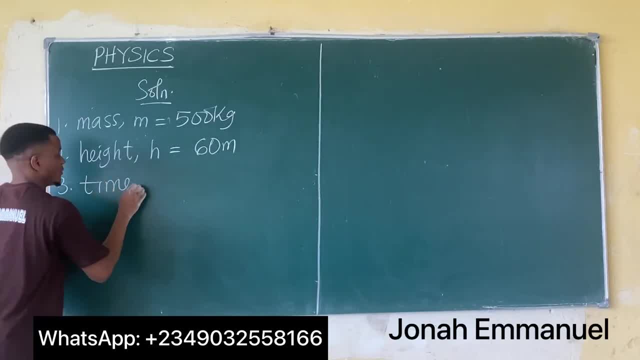 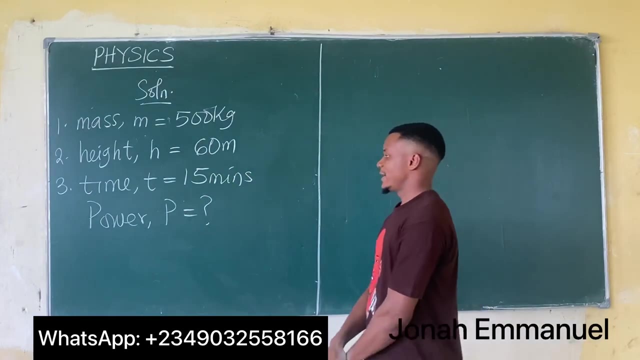 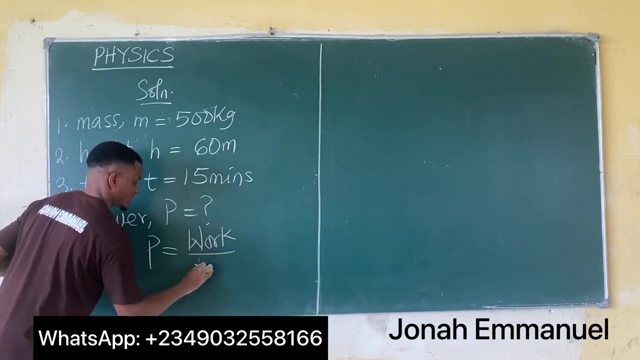 the same in 15 minutes. I'm giving time t as equal to 15 minutes. I'm asked to find power. P equal to unknown. Alright, so first things first. what do I know I don't have? T is equal to work done all over time. Work done is equal to force, times, distance or height, in this case in meters. all over time, That's T. 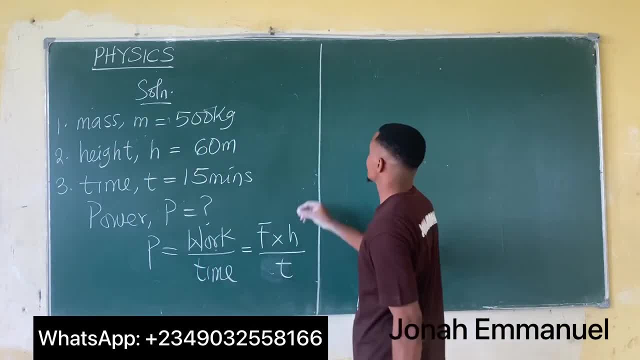 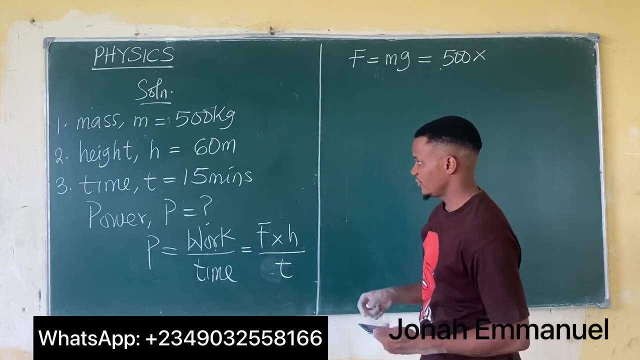 So, first things first, to get force, force is equal to, from using the second law of motion, mass times gravity. That's equal to mass 500 times gravity. Let's see if we are giving gravity as 9.8 or 10.. Let's check. 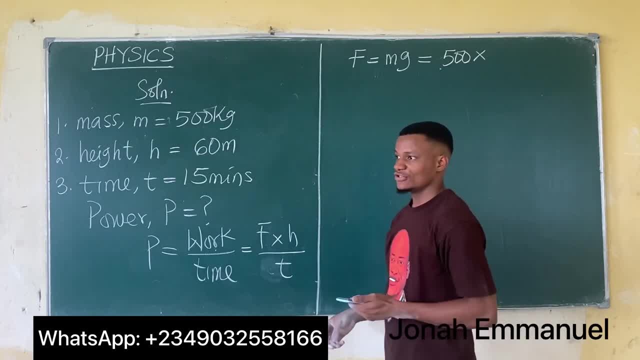 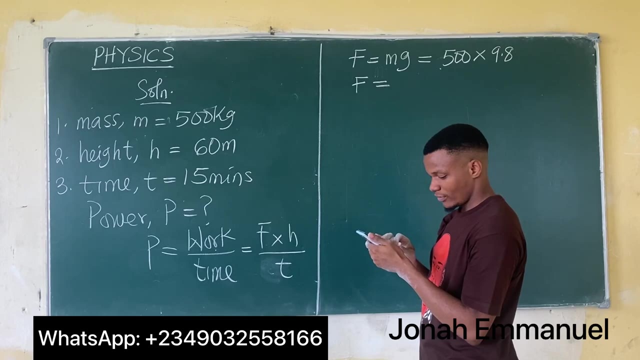 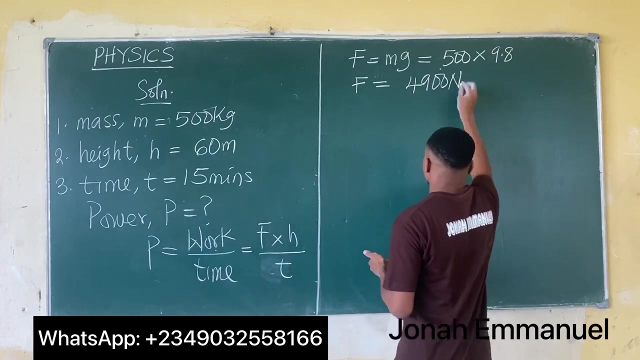 In this question. none was indicated, so I'm choosing to use 9.8 as gravity. Alright, so force F is equal to 500 times 9.8.. We have 500 times 9.8.. 9.8 is about 4,900 newtons. 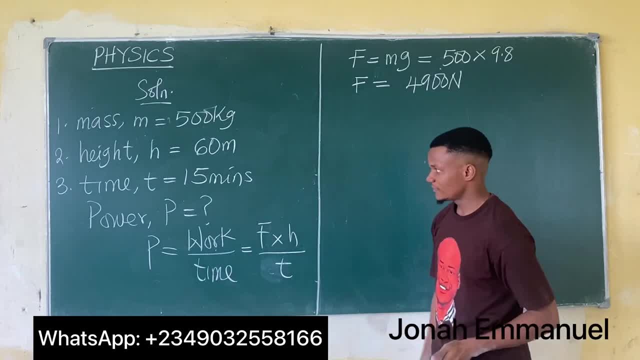 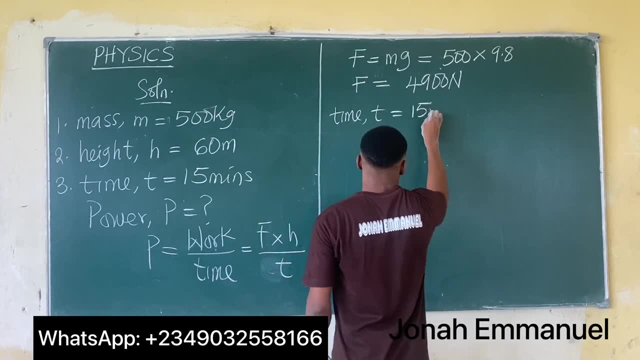 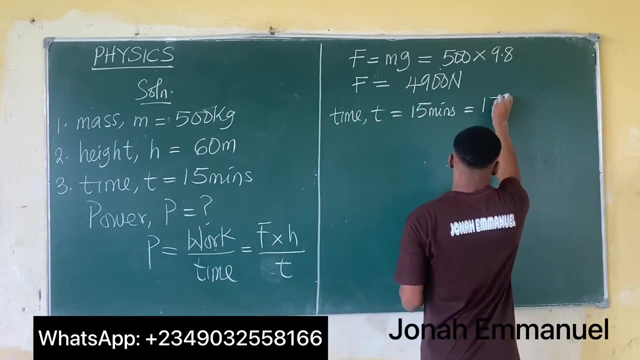 So it's causing the force. The height is 60.. The time is in minutes, So time T is equal to 15 minutes. Convert minutes to seconds. what do you have? Of course you have to multiply by 60. That becomes 15 times 60.. 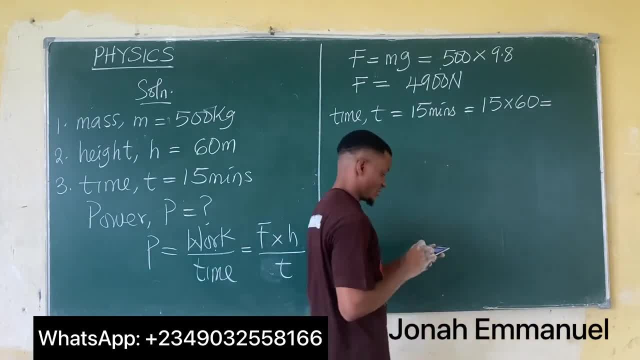 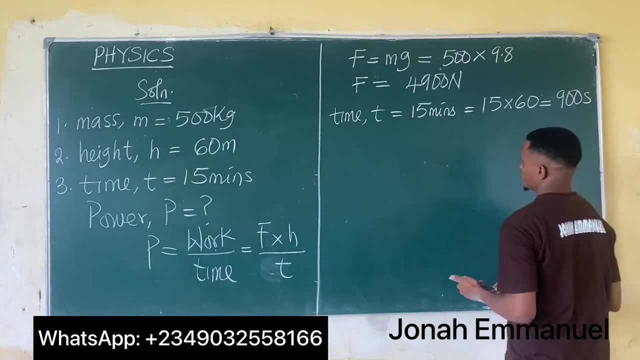 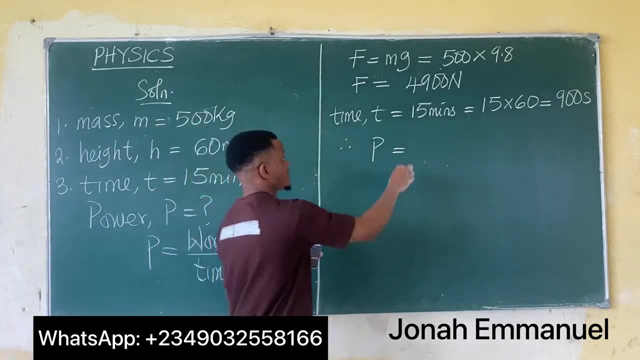 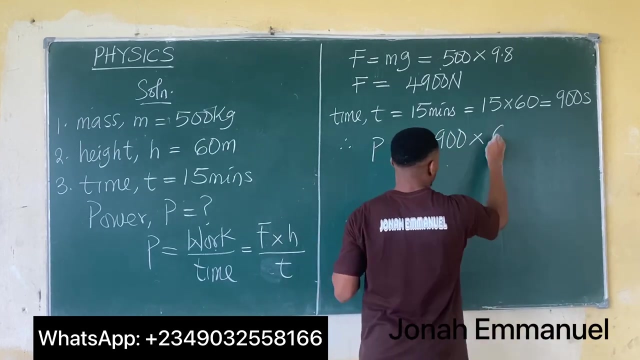 This is how you convert time from minutes to seconds. So 15 times 60, we have about 900 seconds. So therefore the pressure is equal to force. That's 4,900 times height, That's 60 all over time. 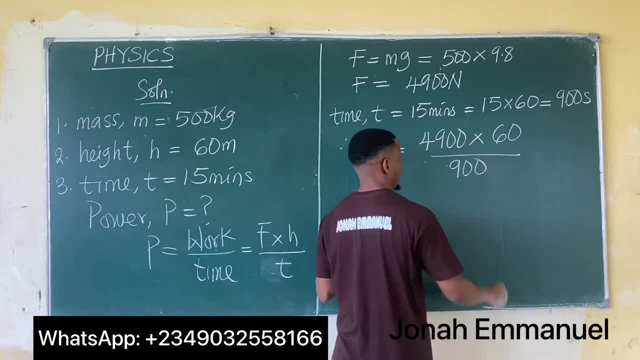 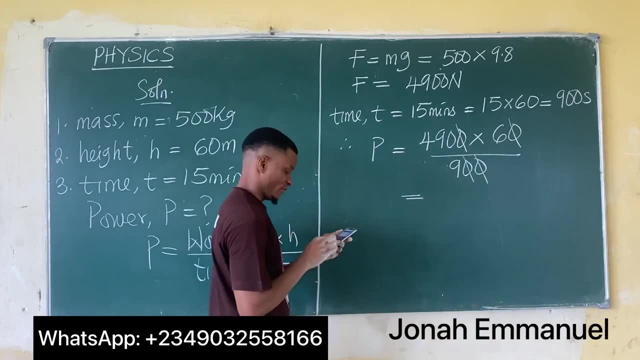 That's 900.. From there, this cancels this, Or you can just do your number by a particular approach. Whichever way you understand, That becomes 490 this times 6.. That's about 2,940 all over 9.. 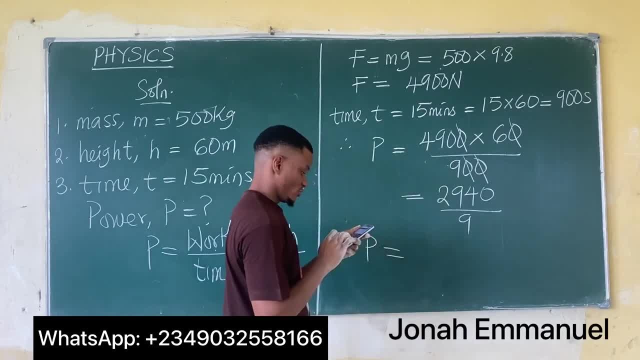 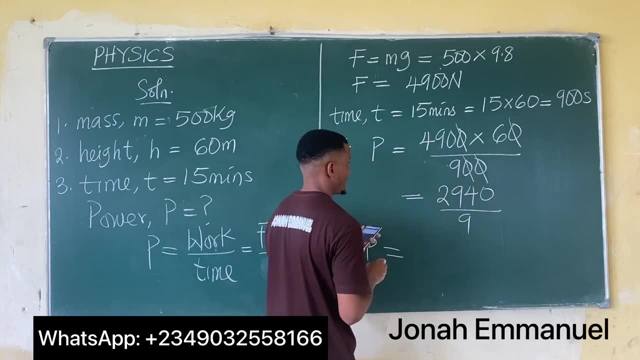 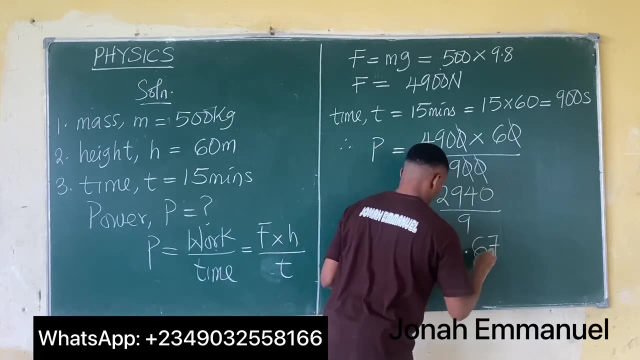 So pressure P is equal to 2,940 all over 9.. That's about 326.67 pressure Or Pa. Not pressure, it's Pa. Of course it's measured in watts. I'm adding this watt. 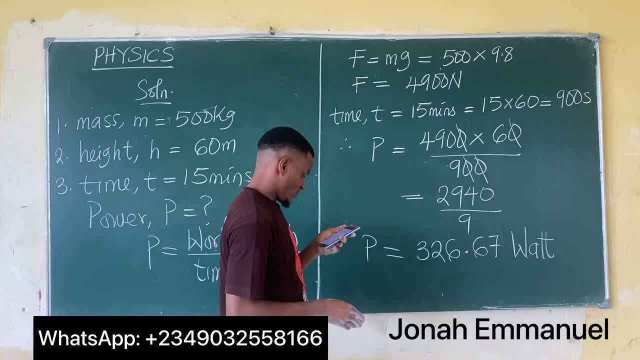 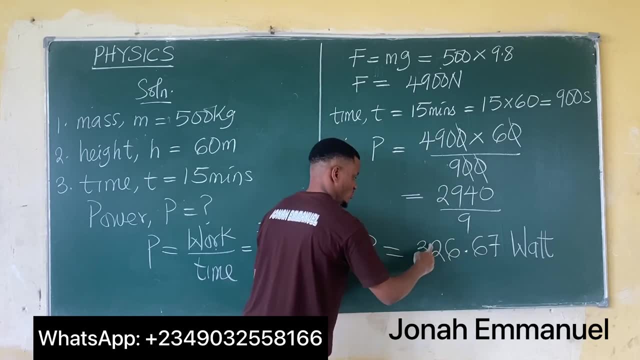 So let's see our options. Okay, So if you look at our options there, From here I'm adding 1,2.. So that's equal to 3,1.. So this should be 3 from here 1,2.. 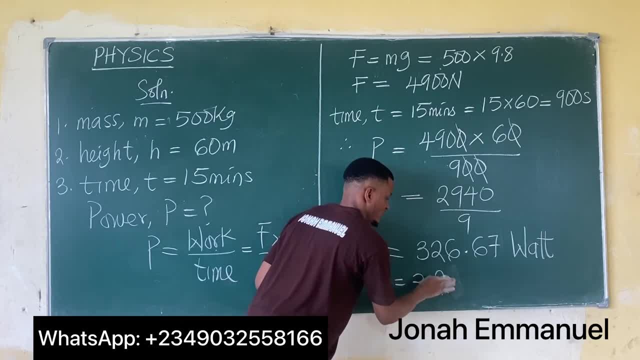 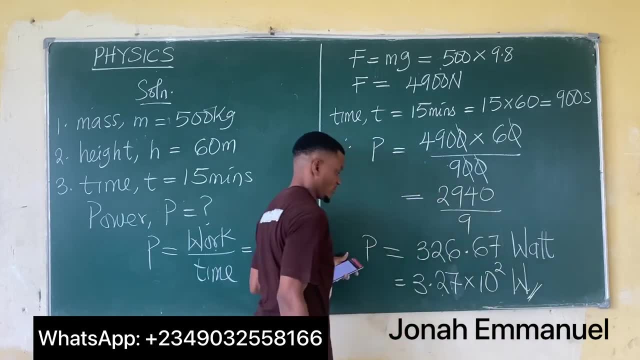 3,2,6.. Or perhaps 2,7.. So my presumption would be equal to 7 times 10, to the power of 2 watts. That's W. But then I'm seeing a presumption towards one decimal place. 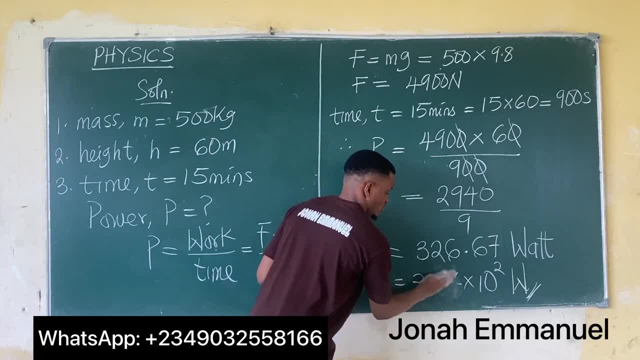 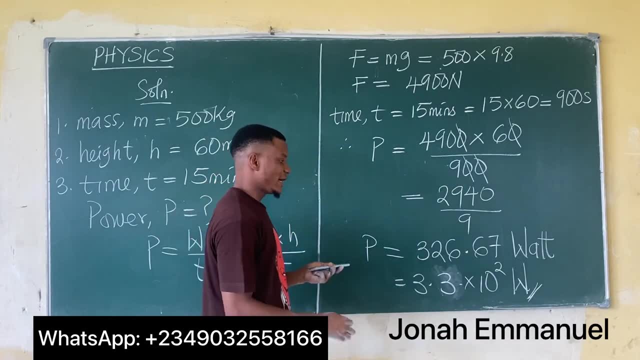 So for this now the one decimal place becomes 3.. It becomes 3,3 times 10 to the power of 2 watts. Of course watts is the same thing as watt. It's the same thing as watt there. Joules per second. 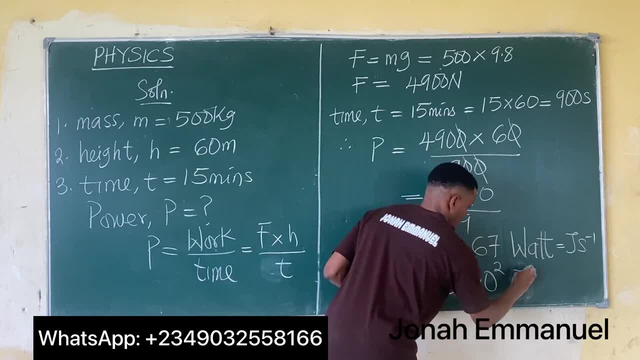 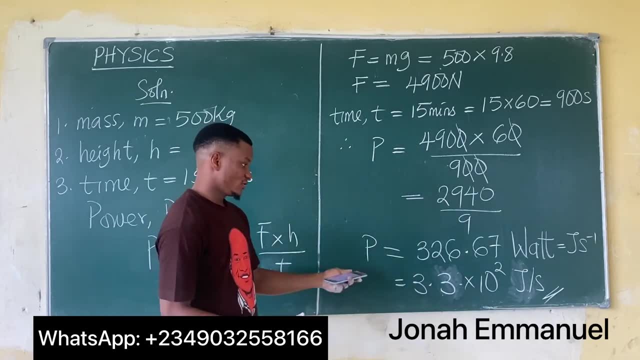 The same SI is So this in joules per second. So joules per second of watts are dimensionally homogeneous. It's the same thing. So hence my answer is 3.3 times 10 to the power of 2 joules per second. 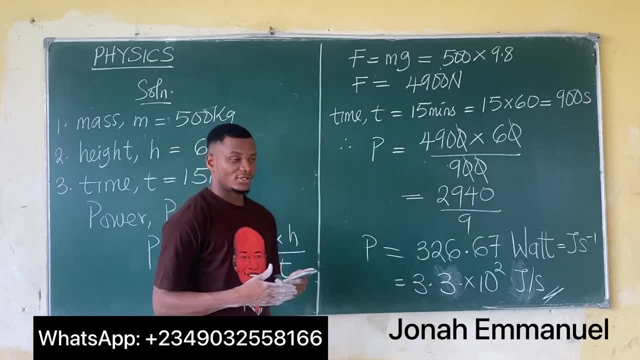 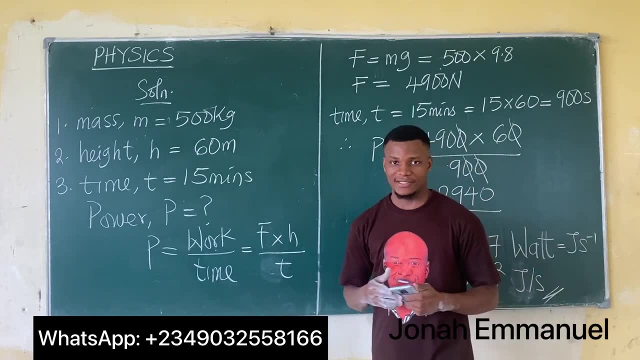 So the correct option. there is option D: Alright, So this is as much as you can take for pressure. See you in the next class, Bye, Bye.